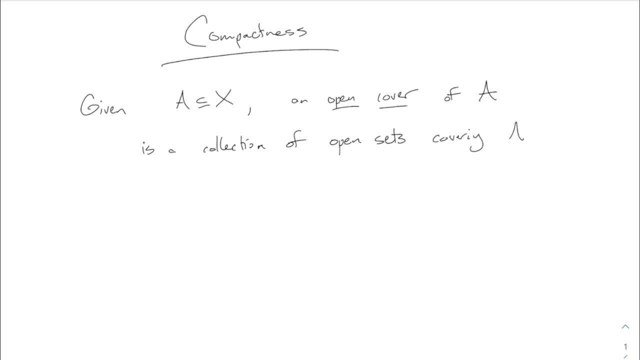 covering A. By covering I mean ie A is a subset of the union. Sorry, I didn't give it a name: Open sets. I'll call it O. Our book uses like a script O, which is why it has the little curly thing on. 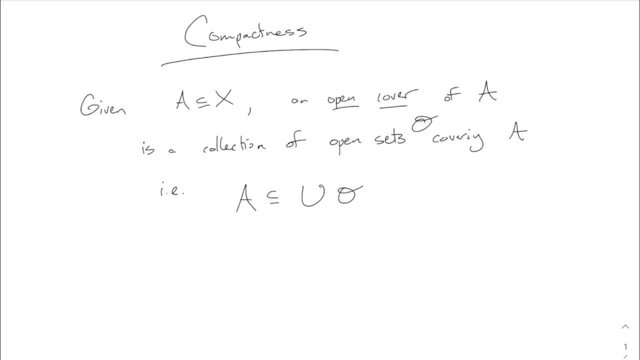 the top. That's my script: O, Such that. sorry, I didn't mean to write the O right there. I meant that A is a subset of the union of all the U's, such that the U's are in O. That's what I mean. 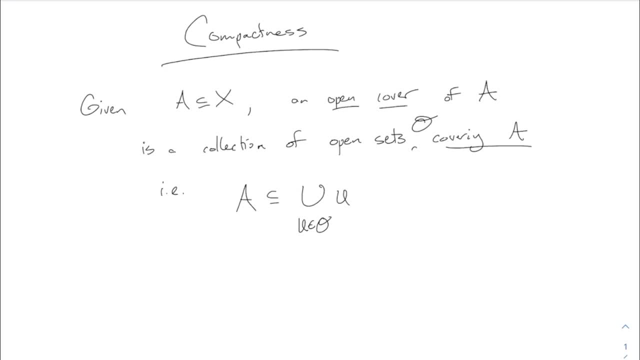 by covering A, that is to say, when you take all the sets from your collection of open sets and union them up, they cover A. So you know, the picture you should imagine is A looks like this and these sets from: 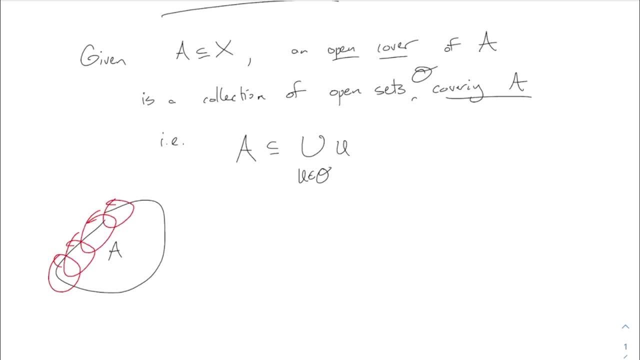 O are all sort of open sets like this that cover everything up. You can make them really big if you want Something like that. That's the. that's a typical picture of an open set. So that's the open cover. It is just a bunch of open sets which cover up all the points of A. All right, Did I? 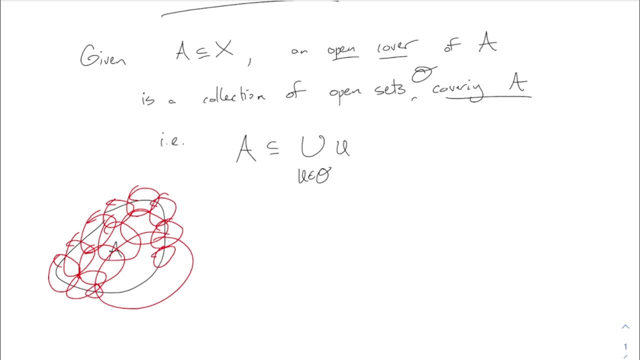 miss one right there, Maybe, Maybe it's a little guy right there. Okay, That's an open cover, And compactness is all about open covers and finite subcovers. So a finite subcover of an open cover. If you start with a big open cover by big open cover, you're going to get a 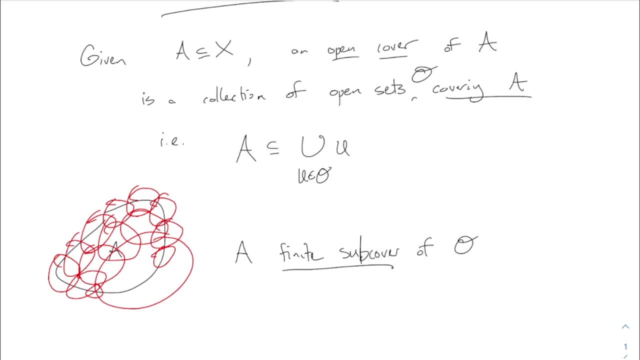 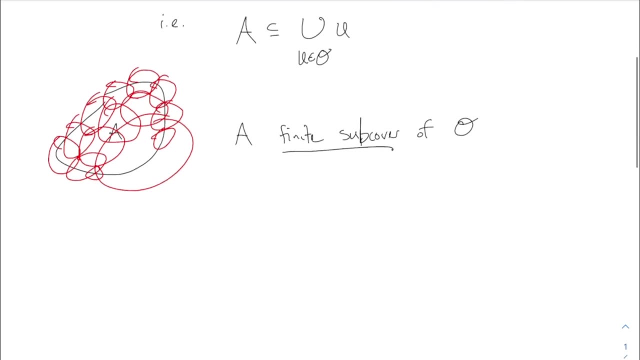 big, I mean maybe it has infinitely many sets in it. A finite subcover just means you pick only finitely many of those things, but they still cover A. So a finite subcover of O is a choice of only finitely many. 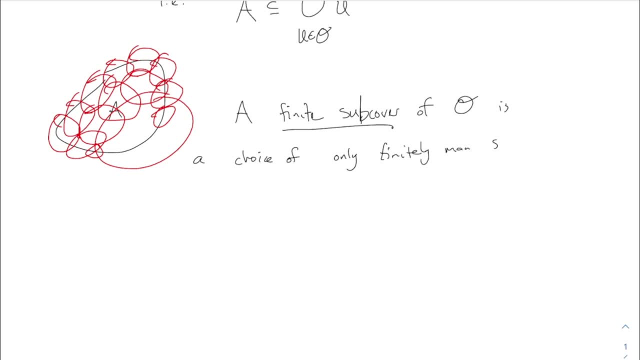 sets in O which still cover A. All right, So A might use infinitely many sets. to begin with, A finite subcover would be: you can choose only finitely many of those sets and they still cover all of A. All right, This may not even be possible. 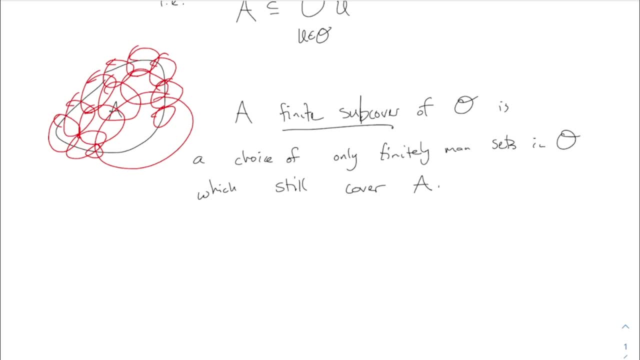 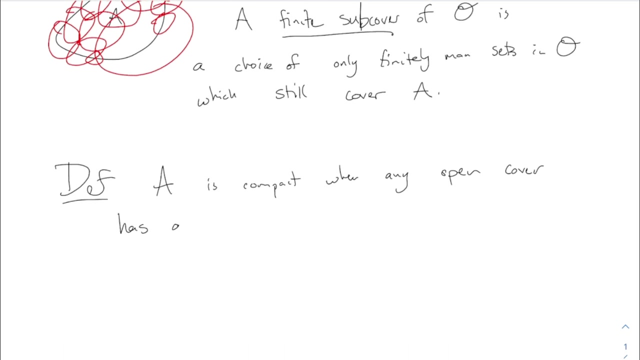 depending on what kind of set you're talking about. There may not be any finite subcover, but maybe there is. All right. And then the definition of compact. we say A is compact when any open cover has a finite subcover. All right, That's the definition of compact. Any open cover has a finite subcover. This 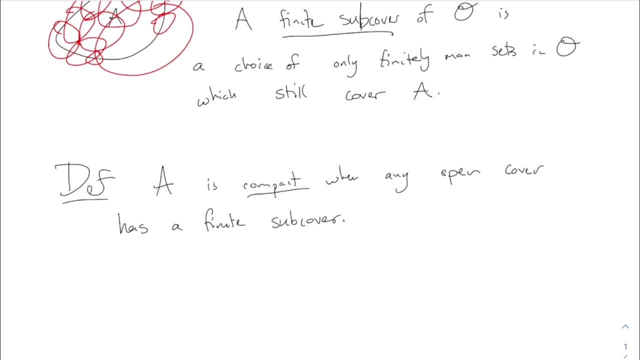 in my opinion, is a very weird concept and it's not obvious at all what this has to do with. anything even like, say, connectedness, I feel like is a very ordinary type of concept and it's obvious why connectedness is important and interesting. I would say compactness is not. 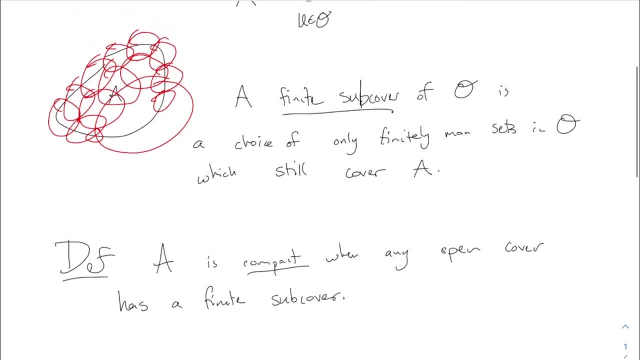 at all obvious why this would be important for anything. It turns out to be extremely important when you're doing topology, And the history of the idea of compactness actually is more complicated than this. People didn't come up with this open cover, finite subcover definition for a long time. 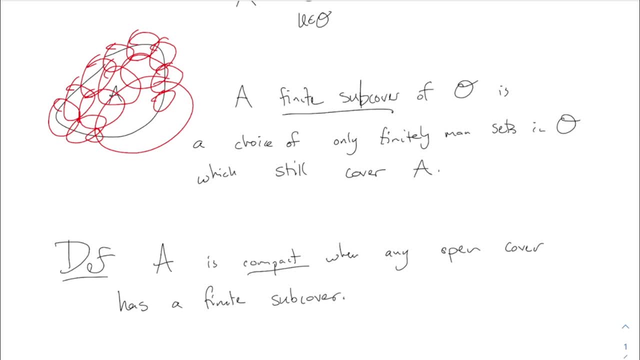 Compactness had been discussed, way you know, far earlier, in terms of like closed and bounded, or in terms of sequences, but it was only after much reflection that people decided that this open, cover, finite subcover thing is actually what's most topologically important about this. All right, Anyway, that's what 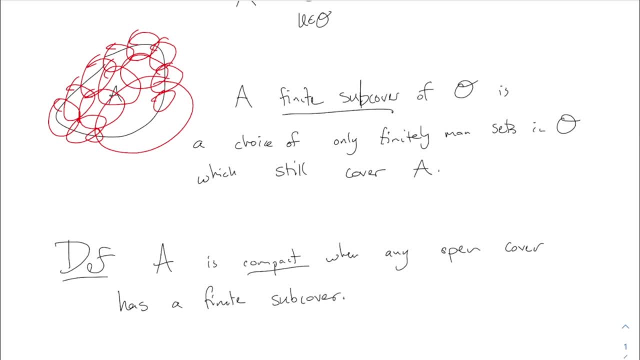 the definition of compactness is. I want to do several examples here and then I got some for you to try of compactness. I want to do several examples here and then I got some for you to try of compactness. 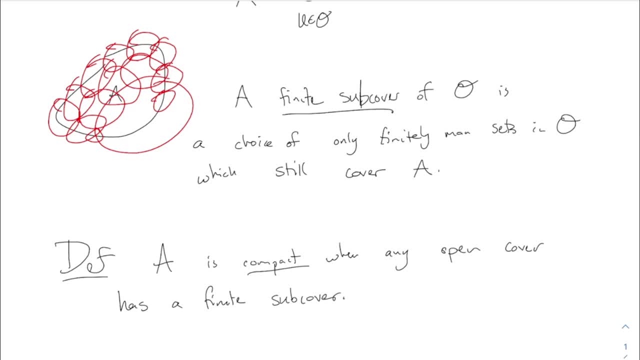 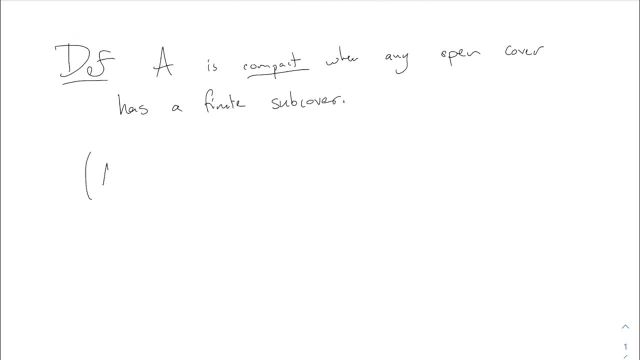 kind of demonstrating that certain sets are not compact. So A is compact when any open cover has a finite subcover. Can I just say A is not compact? This is not really part of the definition, but just What does it mean to be not compact? That would mean there is some open cover, but it 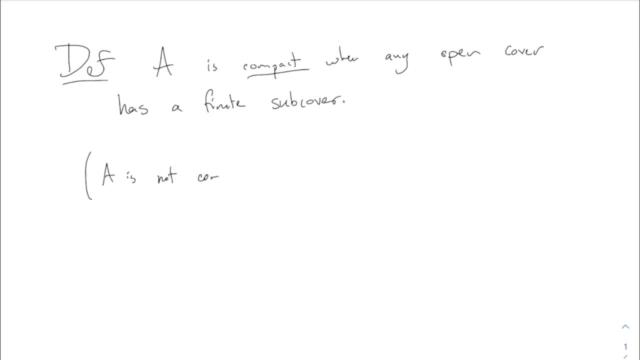 does not have a finite subcover. So A is not compact means there is some open cover with no finite sub cover. right, that's what it would mean to be not compact. what that would mean that would look like something like infinitely many sets covering a. 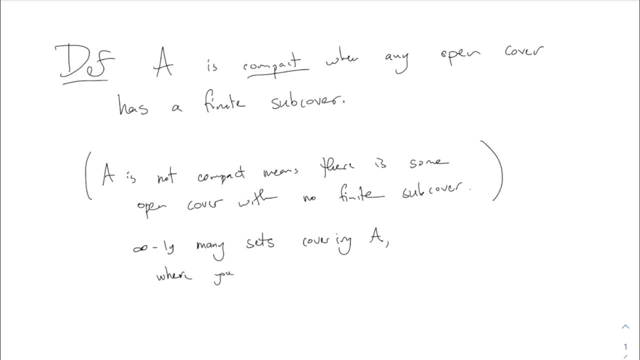 where you really need infinitely many. you cannot just do it with with only finally many of them. infinitely many sets covering a where you really need infinitely many. right, that's what it would look like if your set is not compact. it is. it can be covered by infinitely many sets. but 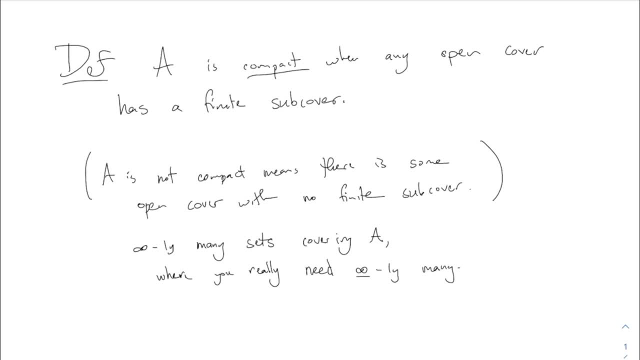 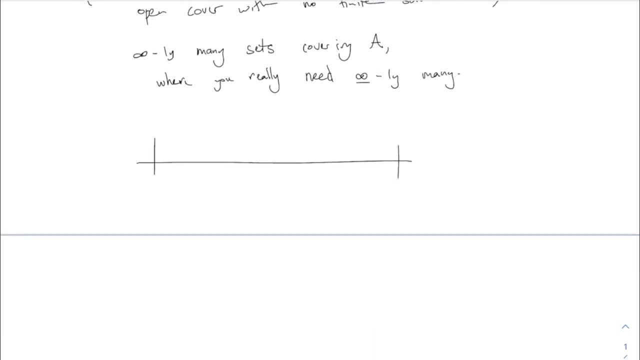 you actually need to use all. you actually need to use infinitely many sets. you can't do it with some finite sub covering, all right. so I think we talked about one example of this last time. that was- I use the example of real numbers. say, a is the set of points. 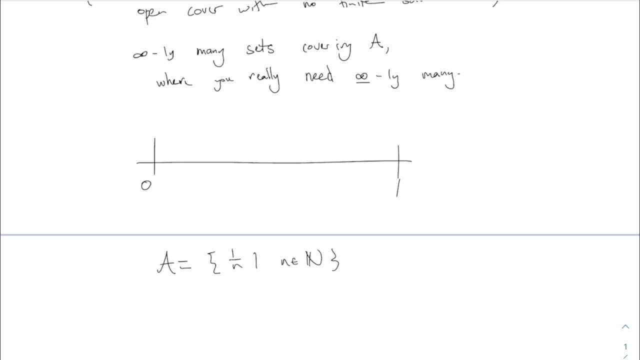 one over n, where n is a natural number. that looks like, you know, one, a half a third, fourth, et cetera. it's these points approaching but not ever reaching zero. and then the open cover that you can use, which has no finite sub cover, would be something like, if I take open intervals: 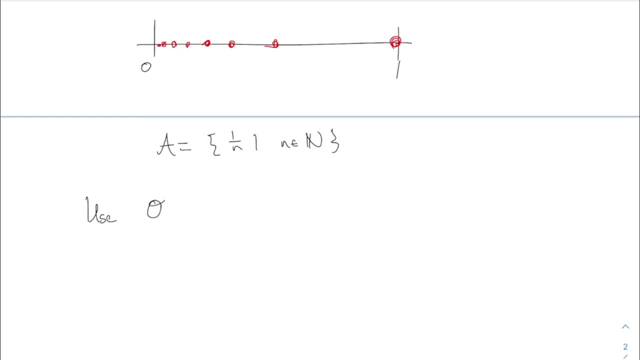 I can use O as the open intervals. if i just take the interval, say 1 over n to to 2. each time I have to. you have to actually cover all these points, but what that would look like is 1 half to 2 is like that, and then 1 third to 2 is like that. 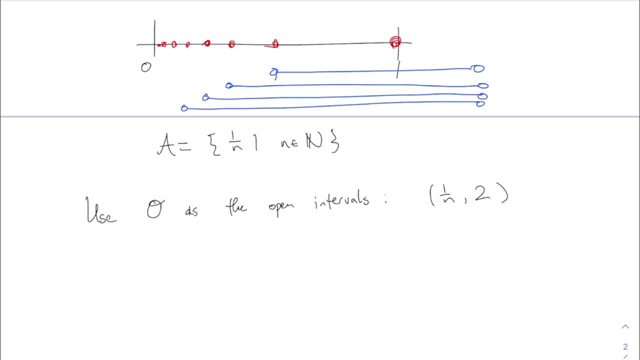 These are my sets from the covering O right. This is 1 half to 2, this is 1 third to 2, etc. And I believe it is true that each of these red dots, eventually is going to be in one of these blue sets. all right, 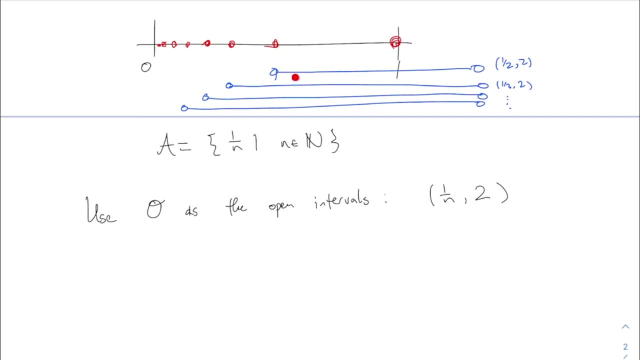 Like this red dot here at 1 half. it's not in this one because I exclude that endpoint, but it is in this one, all right. So these blue guys, they do actually cover up all of these dots. So the open interval is 1 over n to 2, all right. 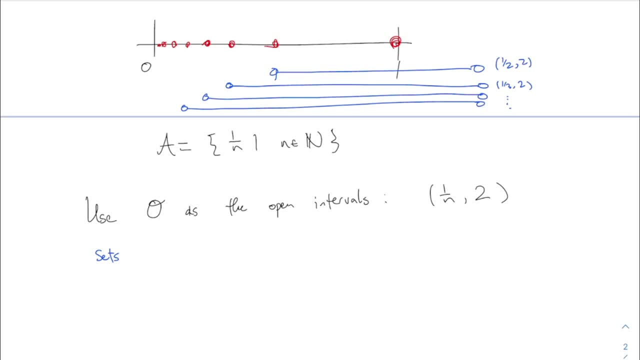 So sets from O- oops, I'm still blue- Sets from O. first of all, they are open sets, right, Because they're intervals and they cover A, Because every one of those red dots is in one of these blue sets. 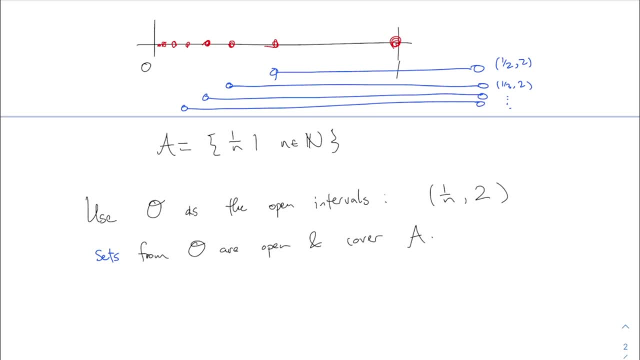 Every one of those red dots eventually lies in one of these blue intervals. But the question is: can I still cover A by using only finitely many of these intervals? Is it only like maybe I only need like 4 of them, or something? 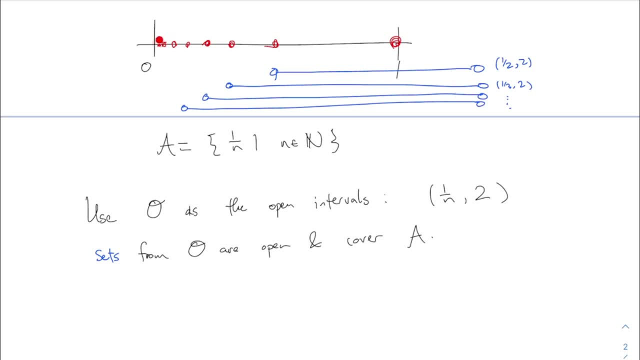 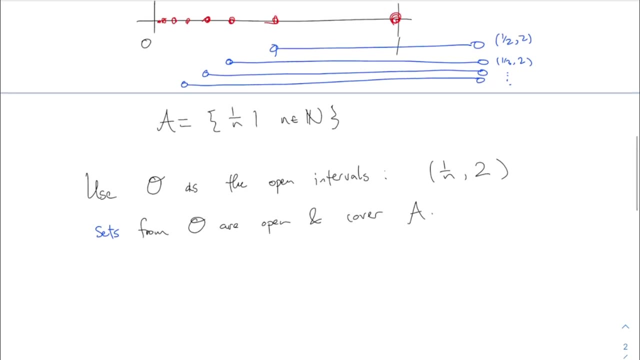 The answer is no. If you take only finitely many, you're always going to be missing some of the points that are close to 0. So these guys here have no finite subcovers. So sets from O are open and cover A, but 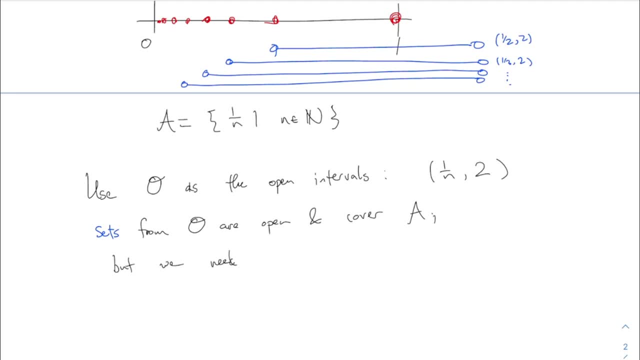 We need infinitely many to cover A right, Because no individual one actually stretches all the way and gets all the points. So that means so this O that I said has no finite subcover. So that means A is not compact. This is an open set. 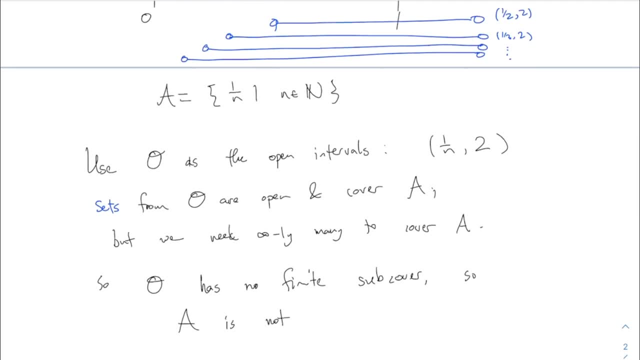 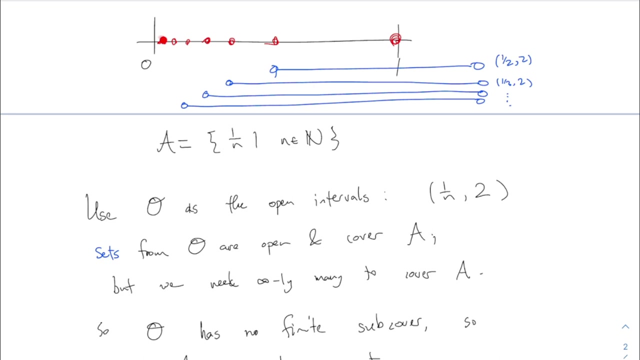 This is an open cover with no finite subcover. All right, I hope that that makes sense. There's actually a kind of a strategy that I used to choose those intervals. I chose these intervals so that they would sort of stretch out in a way which approaches where these points are also approaching. 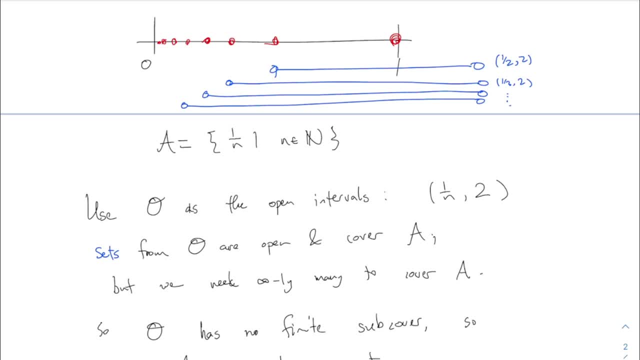 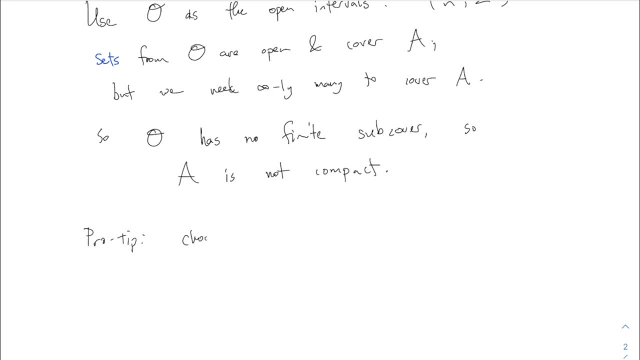 That tends to be a good idea. Yeah, So this is a very vague bit of advice, but here's: my pro tip is to choose open sets that are somehow like stretching out to the boundary or something like that, Something like that. 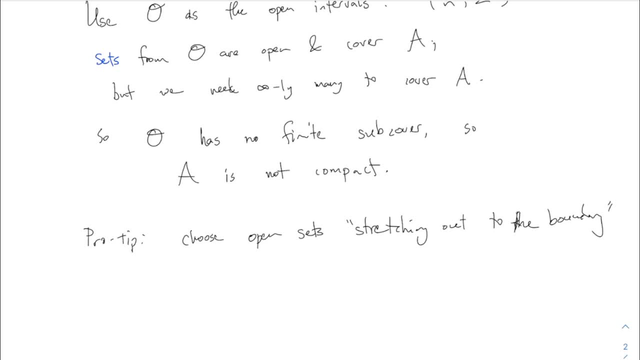 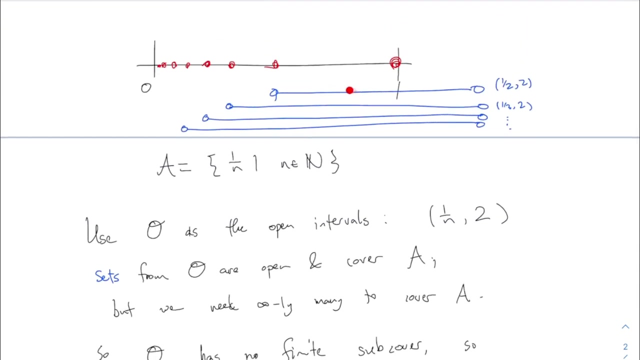 Choose open sets which sort of gradually approach the edge or the boundary. This is vague advice, And you have to know what you're looking for, which comes from practice. But, for example, why did I make them stretch towards this end, the left end rather than the right end? 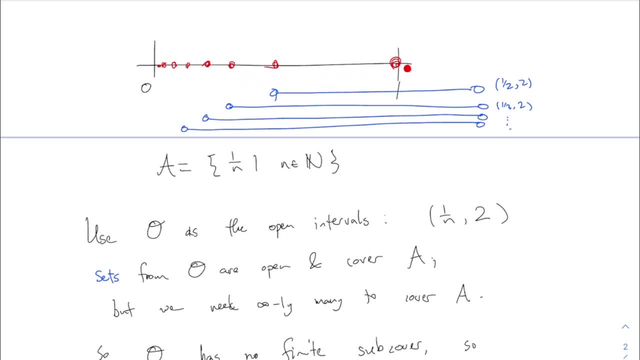 Well, I think you can tell If they stretch towards the right end. there's only one point there, So you don't actually need infinitely many things if you're trying to stretch them out towards the right end. But if you're stretching out towards the left end, then you do have this issue with there being infinitely many things over there. 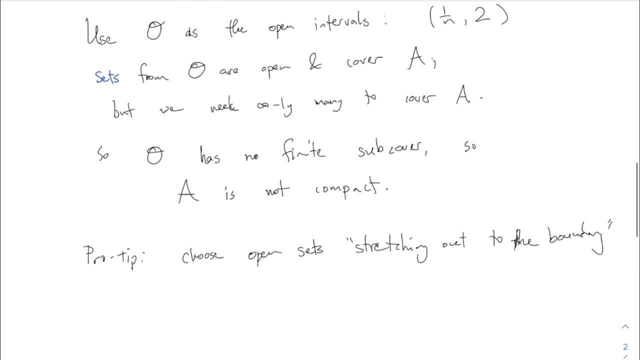 So there's some amount, There's some amount of practice that it takes to kind of see what you want to do. All right, This is my basic example. Let's try some more examples And then, like I said, I've got some for you to try out. 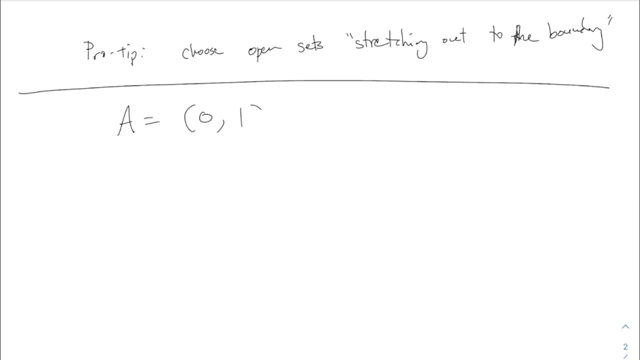 How about this? set Just the open interval 0 to 1.. Is it compact or not? It is not. I'm here to tell you, This is not compact And I want to do a similar kind of thing. Okay, So what does it take? 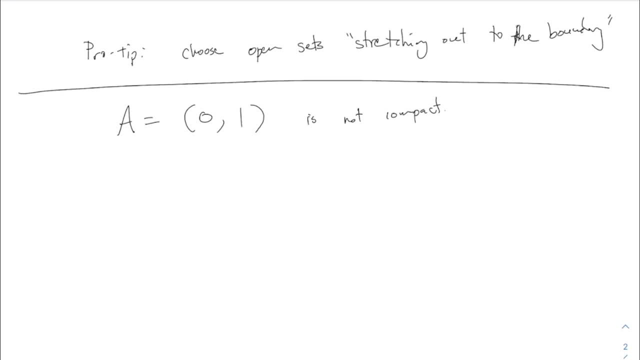 To demonstrate this, you have to tell me an open cover which I'm going to just use intervals in this case. You have to tell me an open cover which has no finite subcover, So I'm going to say, let O be the cover, using intervals like: 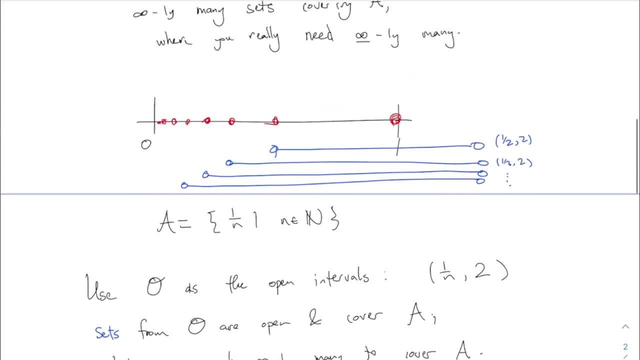 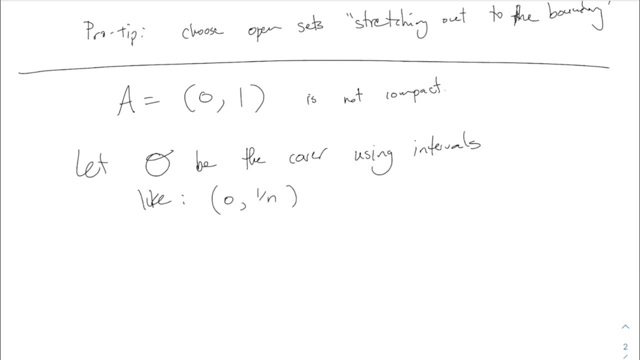 Actually, the same intervals from here can be used in this same example, But just to make things a little more interesting, how about I will use a slightly different one? How about just 0 to 1 over N? All right, So in this example, my entire set is this open interval. 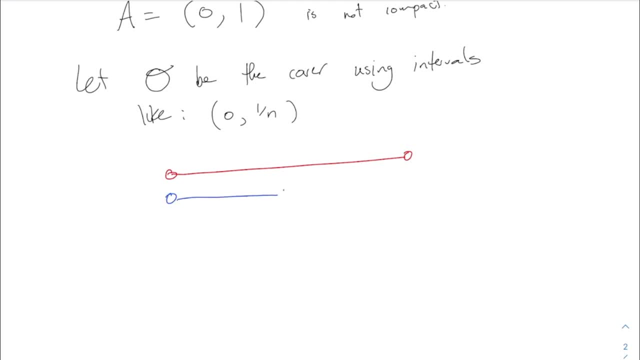 And the open cover I am using takes intervals like this. I didn't mean that 0 to 1 over N, That's not a. I did mean that, Did I? No, I didn't mean that. If it's 0 to 1 over N, can I just say: how about this? 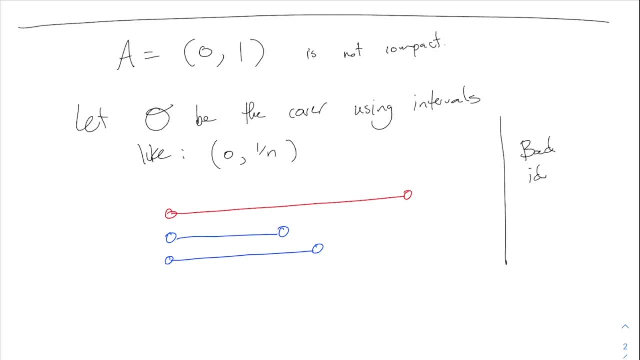 I totally meant this as a bad idea example. Sometimes you got to do bad idea examples right. What's wrong with this example? The open cover. the first one would go all the way, 0 to 1. And then the next one goes only halfway, then only a third of the way. 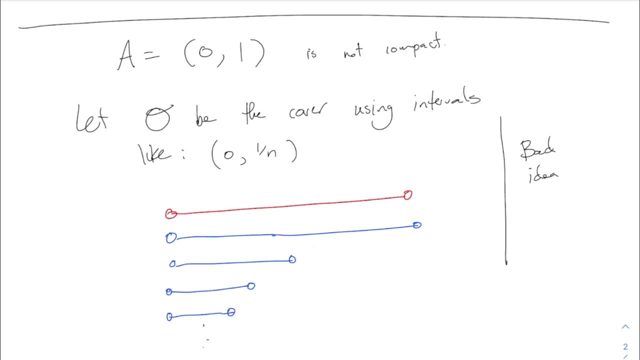 then only a fourth of the way, et cetera. right, And now I say something like remember, the point of this is that all these sets together cover up the interval. Actually, that's true. If you look at the union of all of these things, you do get the whole red line. 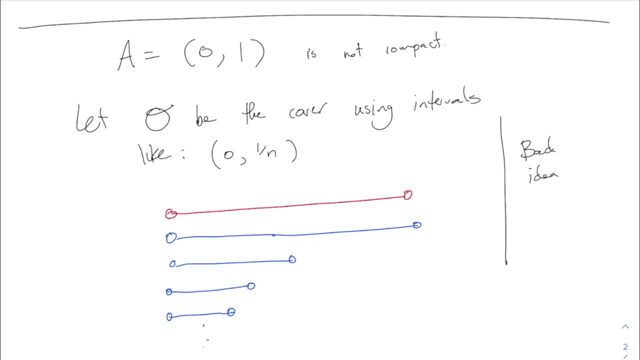 Do we actually need all of them to cover the whole thing? And the answer is no. That's why this is a bad idea example, Because actually you only need the first one, right? The first one all by itself already covers the whole thing. 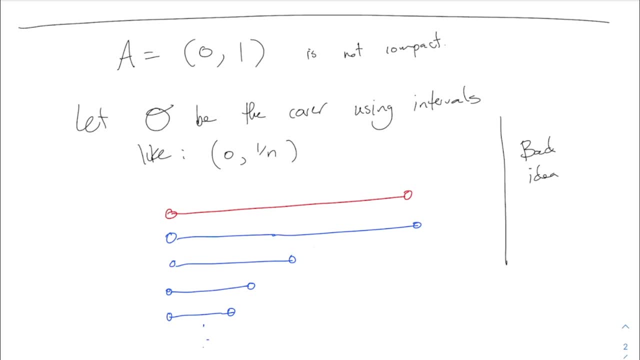 So is there a finite subcover? The answer is yes, I can still cover it. I'm using only one of them, And so this is not a good choice of the open cover. So this one, this has a finite subcover. 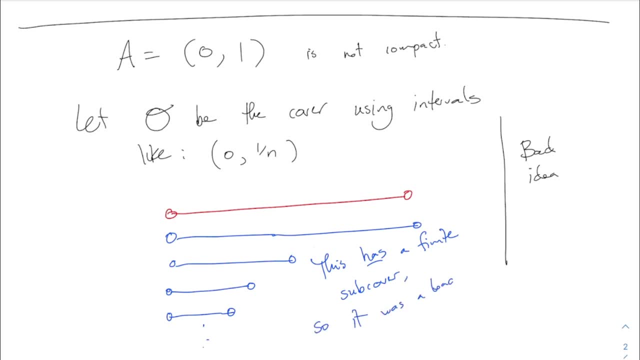 So it was a bad choice. Does that mean it's not compact Or does that mean it is compact? I'm trying to show that it's not compact. If you say it is compact, it means every open cover has a finite subcover. 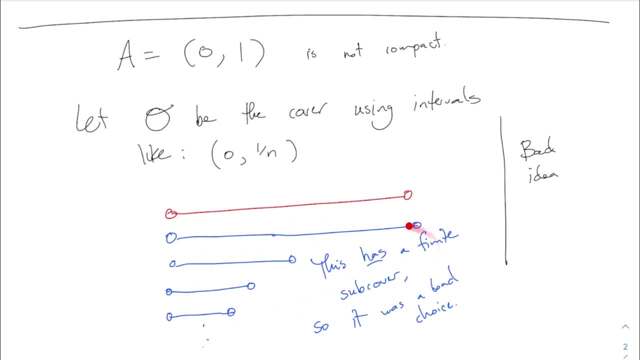 Just because I showed you an open cover which has a finite subcover doesn't mean that it is compact. It just means that was perhaps a bad choice of the open cover. Anybody see how could I modify this? This is actually not what I meant. 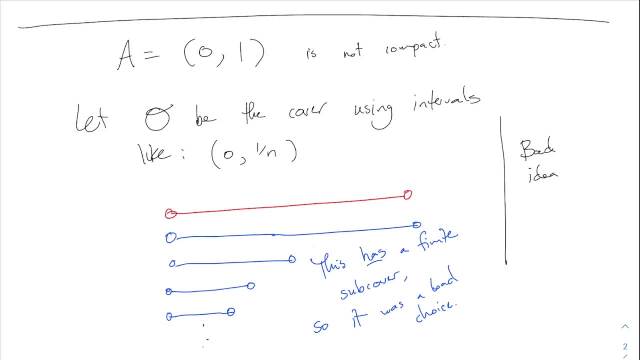 You want to make it so that they gradually stretch out, eventually filling up the whole thing, rather than I had one that already filled up the whole thing and I shrunk it down. That's the wrong idea. One minus one over n Zero to one minus one over n. 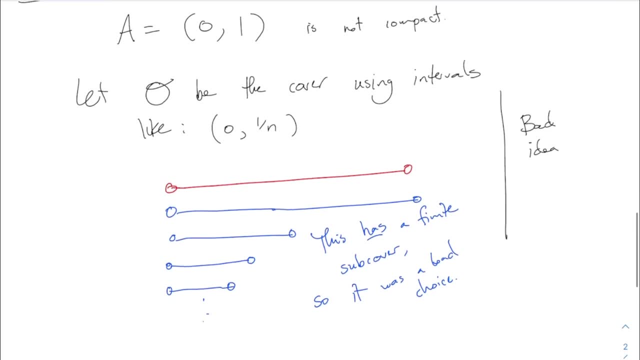 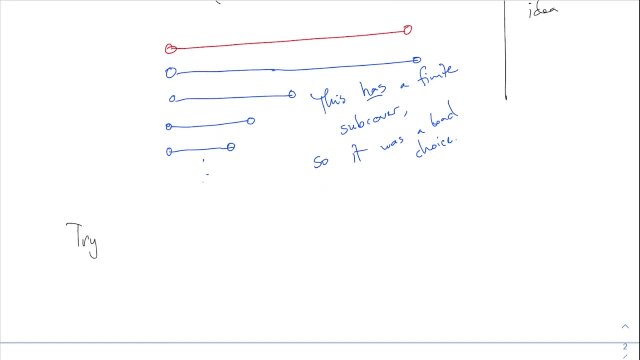 Yeah, that's great. So let's start, Let's try instead. So all of that was a not entirely bad idea. How about let's try? if I were to write specifically the interval zero to one minus one over n? Yeah, Where n is a natural number. 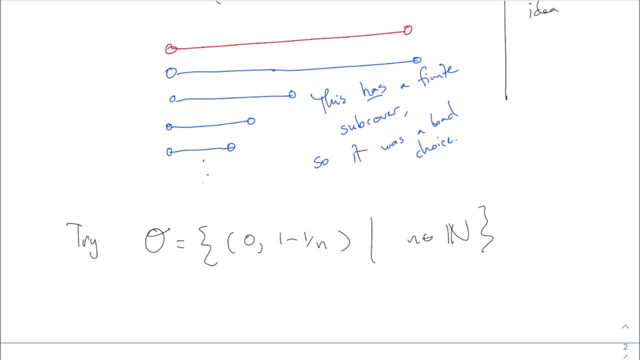 Here I wrote O as a set. Remember, O is a collection of all of these intervals, So you can make it a set if you want to. It is the set of all intervals that go from zero to one minus one over n. Now the picture. 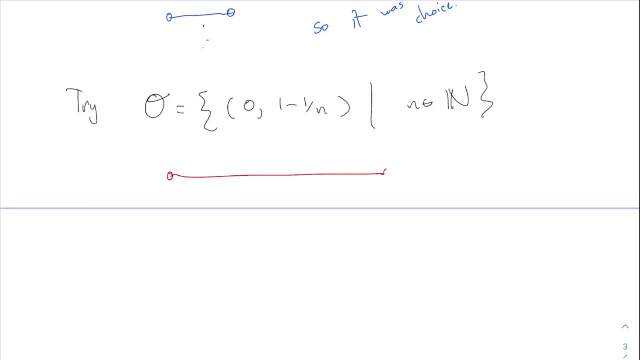 This is what I meant to say the first time. Now it looks like first one would be actually zero to zero doesn't make a lot of sense, That's nothing. The next one goes zero to a half, then zero to two thirds, then zero to three fourths, et cetera. 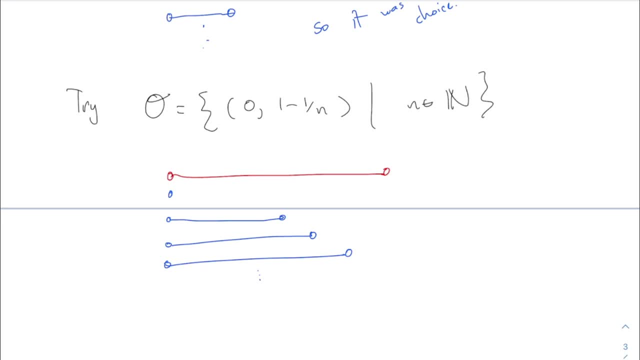 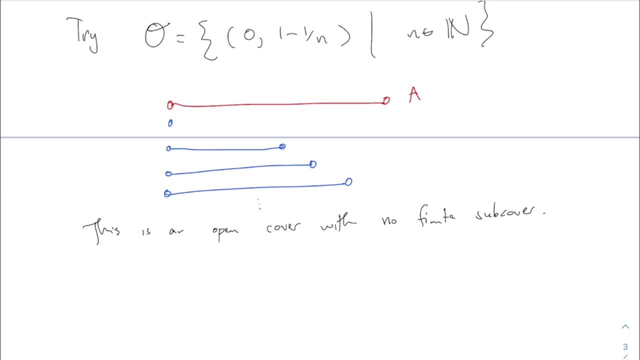 And now it is the case that these intervals, they do fill up the entire original set, Which was A- you know this open interval. So this is an open cover With no finite subcover. Excellent, Any thoughts about that one? 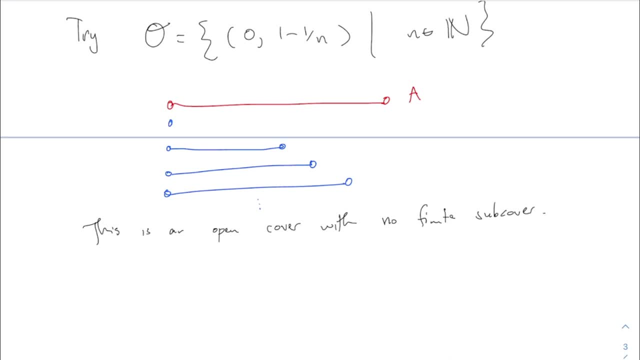 This is an open cover with no finite subcover. All right, What about if it was the closed interval? If that A Instead of an open interval was a closed interval, Can you do a similar kind of a trick with that? So what about? 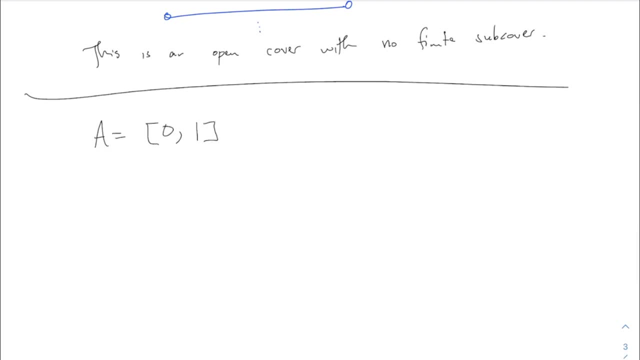 How about A? is the closed interval zero to one? All right, So that's this. I'm trying to write A in red. That's this Now I could Remember. it has to be an open covering, So the sets that you use here, they have to be open sets. 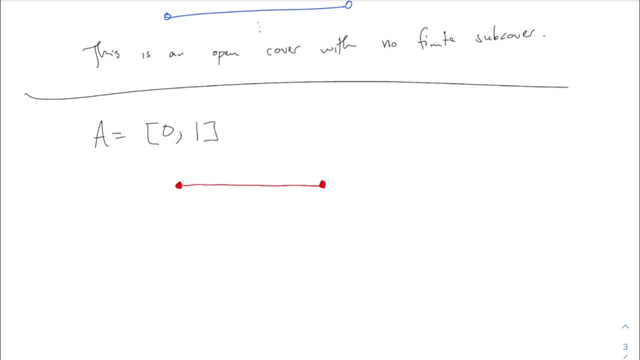 All right, Which is going to complicate matters A little bit. There are a few ways you could try to modify the previous approach, though, So one way would be I could just do this thing. This is what we did before, right? 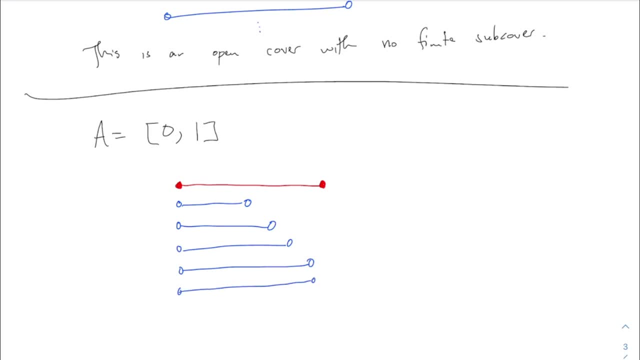 Eventually like approaching but not getting to that point. This actually is not a legal open cover. Can somebody say why? What's wrong with that? Just using the same thing from before? Yeah, this doesn't cover this point And also it doesn't cover zero. 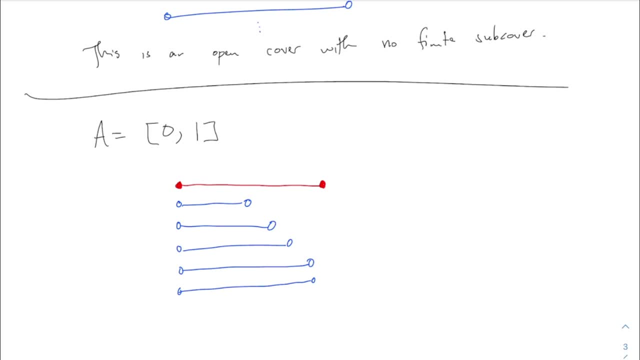 Now I could easily make it cover zero by just moving everything slightly to the left. So that would you know. originally this looked like zero comma one minus one over N. right Now I could just change this zero here to something like minus a half. 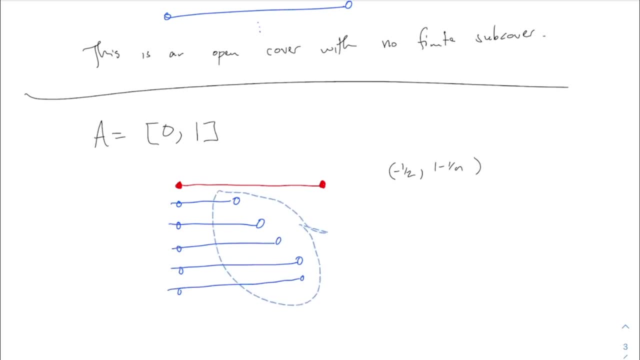 That would basically push all of these guys over a little bit. What I missed? that I was trying to be cute and it didn't quite work like that right Now. it covers zero, but actually it's not going to cover this point. 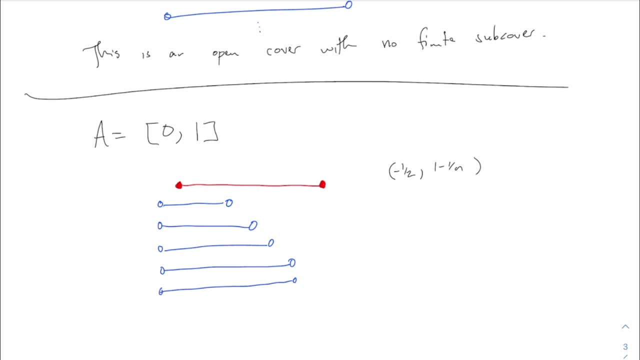 How could we fix that? Anyone have a similar trick? Maybe I could push the right endpoint to the right a little bit. I just tried to slide everything, make it stretch a little bit further to the left. I don't know, I don't know. 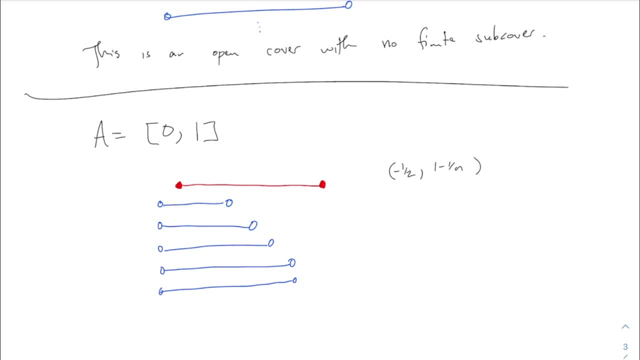 I could also make it stretch a little bit further to the right. Maybe this: instead of one minus one over N. how about let's try maybe minus a half to three halves, minus one over N. That makes it so that these guys actually do stretch. 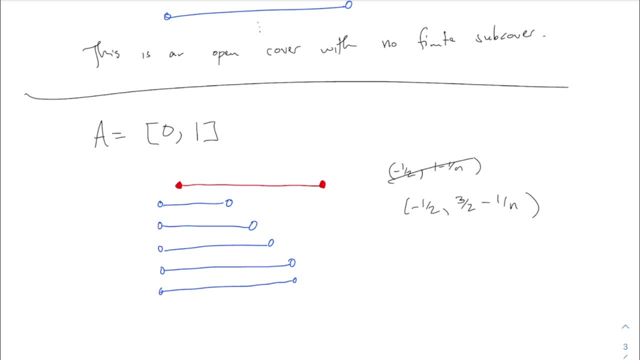 Eventually they do stretch beyond one because they are going to approach On the right side. they approach three halves, All right. So what that would look like is these blue sets now, Eventually they will go past there And then just continue eventually approaching three halves right instead of approaching one. 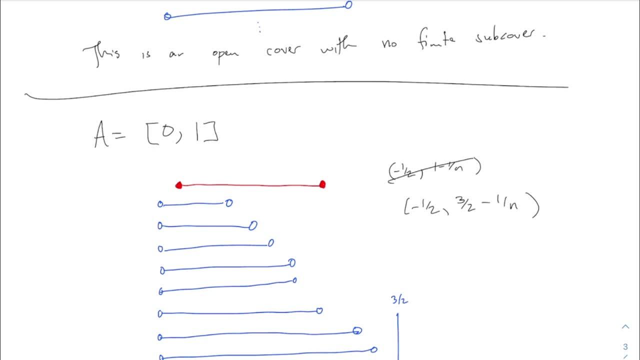 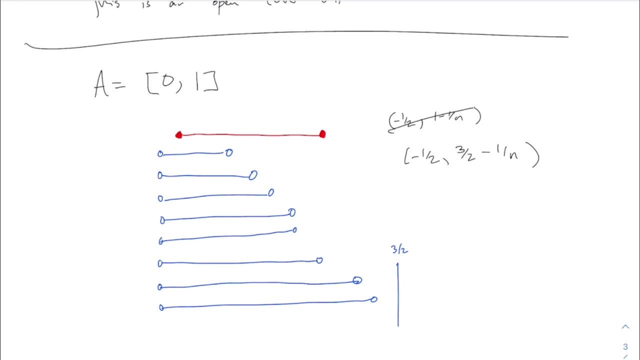 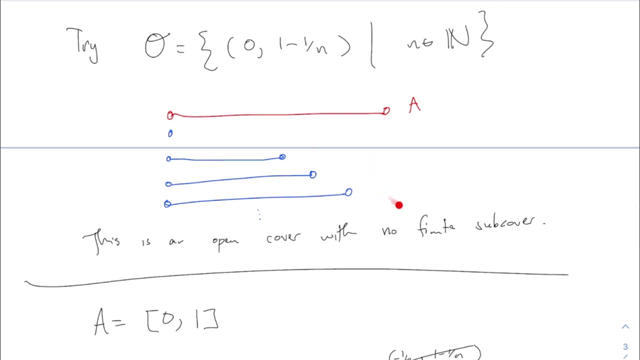 Is there a problem with that? Yeah, you should be concerned about the finite sub-cover business. Remember, the whole point of choosing these intervals here is you actually need to use infinitely many of them because you need it to stretch all the way to the end. 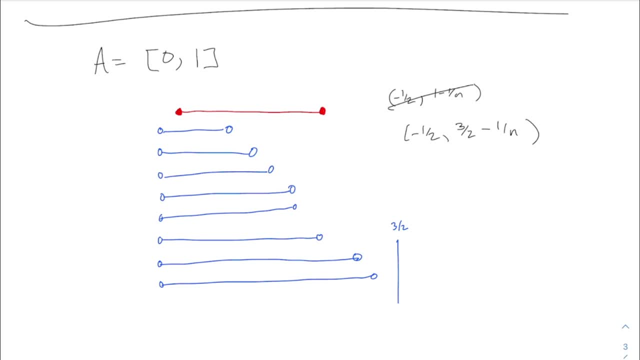 Do I need to use infinitely many? I think you don't, Actually, at a certain point. I mean, on my picture it looks like this one. actually this one already includes everything right, And so you don't even need any of these. 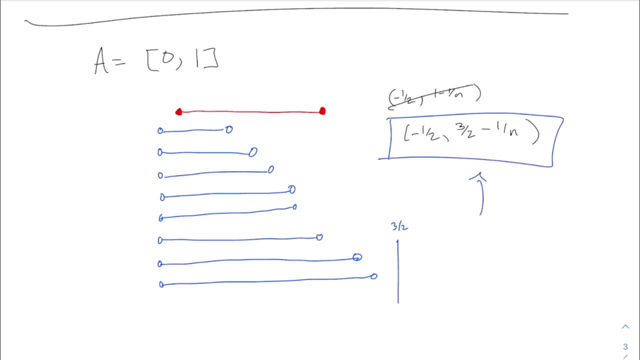 So this covering here, this one, actually has a finite sub-cover, because eventually you get to, if say N is four, it's going to be minus a half comma, three halves minus a fourth, And that already includes the whole interval zero to one right. 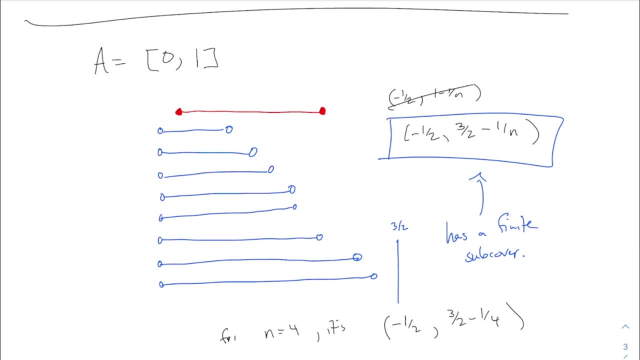 Three halves minus a fourth is one and a fourth whatever. that is five-fourths. That already includes the whole thing. So you don't need infinitely many of them, You only need this one, just one of them. So the unfortunate answer is: this whole thing was a bad. 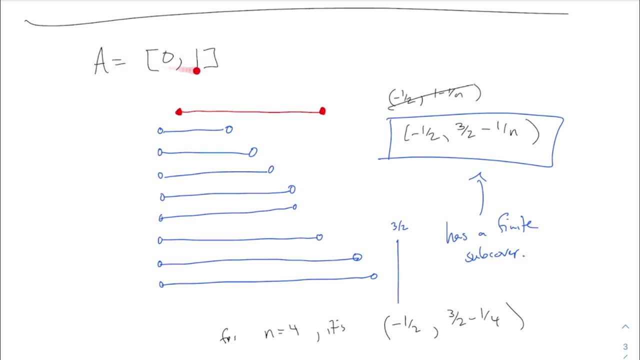 It's a bad idea and it's because actually this is compact, So it's a fact. It's not easy to prove, but we'll get to it eventually. But this set actually is compact. Any open cover you can choose will automatically have a finite sub-cover. 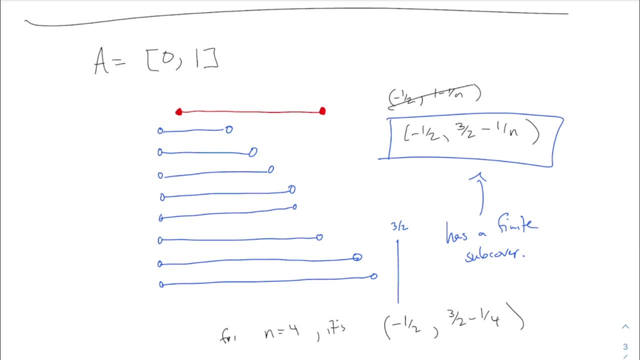 This is not obvious in my opinion, But I mean, if you try and play around with these intervals, you will eventually give up and realize that you probably can't do this in any way. So I'm going to say actually A is compact. 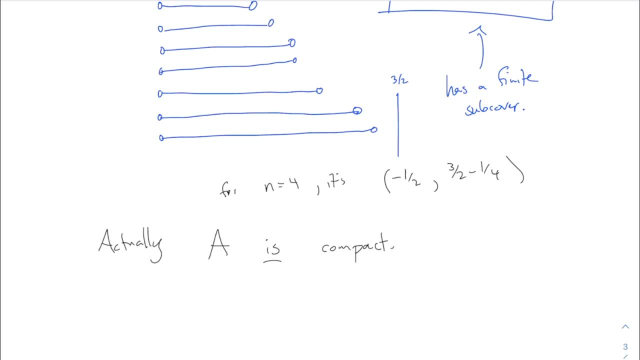 I said, it's hard to prove, although if you remember anything from real analysis, compact is equivalent to closed and bounded, And A is a closed interval and it's bounded. So I suppose you already knew that it is compact. That means this game that I'm trying to play with the finite sub-covers actually is not possible for that set because it is a compact set. 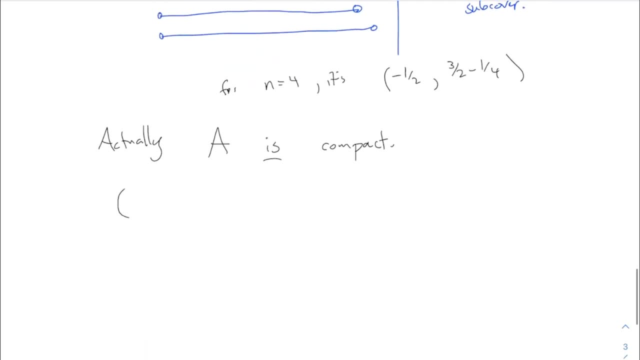 All right. So can I just say this is hard to prove. If you know the Heine-Borel theorem, you say it's closed and bounded and that's it. But this is hard to prove using covers. You would need to somehow need to prove that all open covers have a finite sub-cover. 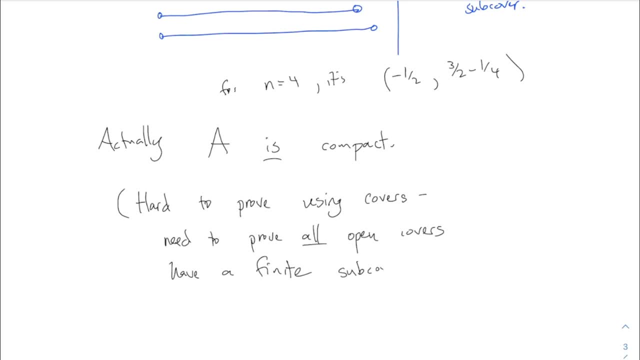 And that's not easy to do. All right, Because you have to somehow imagine, You have to imagine any possible way of covering this up with intervals and then argue that you would require infinitely many of them. Okay, Let's just try a few more. 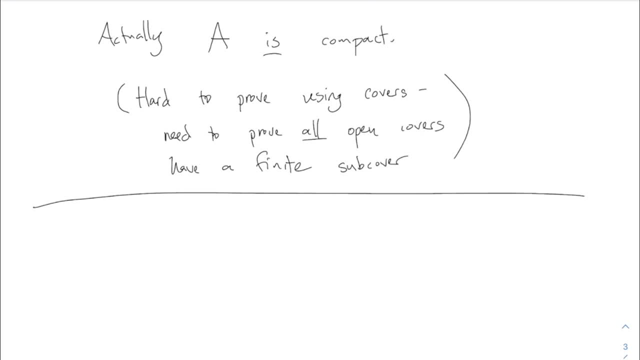 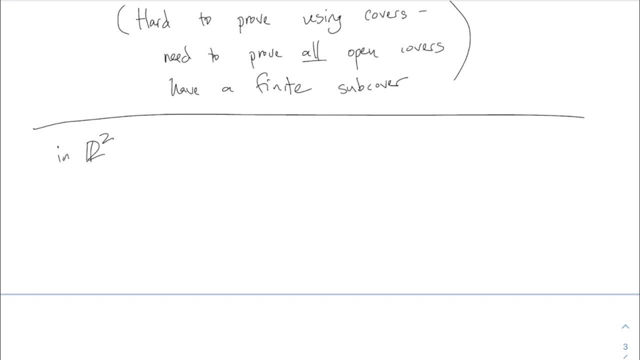 So that one is compact. so you can't say you can't find this open cover with no finite sub-cover. How about in more interesting settings? How about in R2, the x-axis, X-axis. So that's this set here. 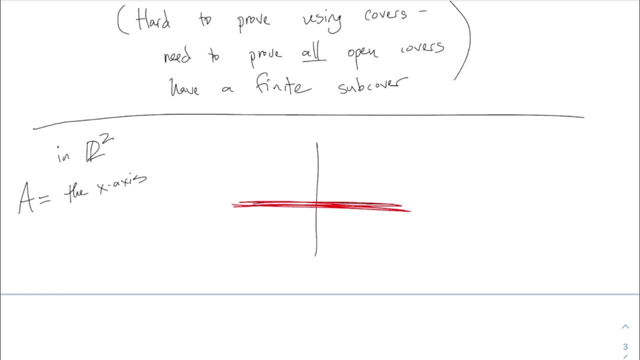 Can we make an open cover with no finite sub-cover? Oh sorry, I skipped an example that I wanted to do. That's all right, I'll come back to it. Can I make an open cover with no finite sub-cover? Now, I've been using integrals. 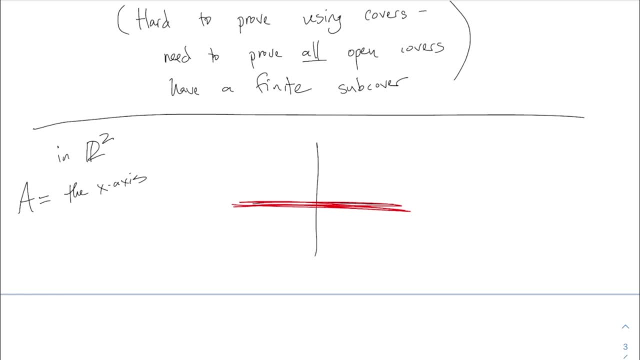 Intervals in the other examples, because that's what open sets in R look like. I'm talking about R2. now The sets that you use should be probably balls, open balls which look like circles, Or I mean you could. there's some cases when you want to use other, weirder looking open sets, but you might as well. 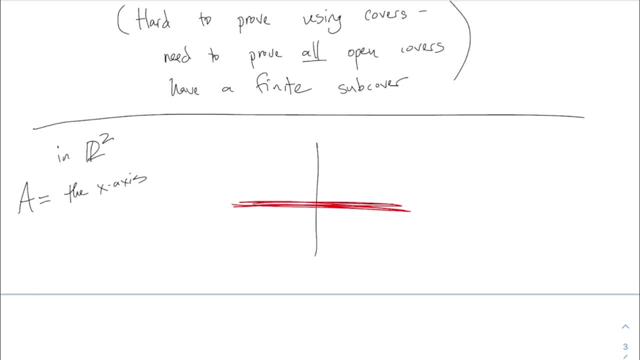 Can anybody think of a way to choose, cover this up with individual balls, little, you know, circles, They don't have to be little, They can be big if you want, So that you actually The idea is, you make these balls, I said make them stretch out to the edges somehow. 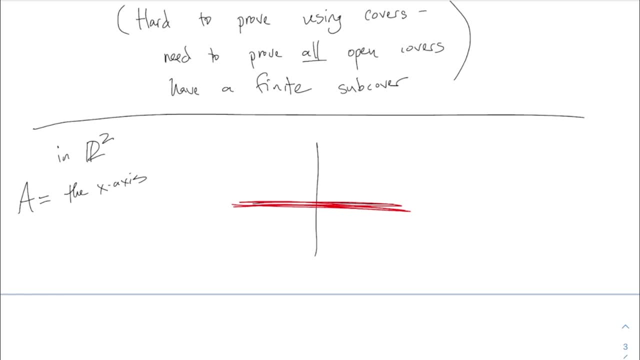 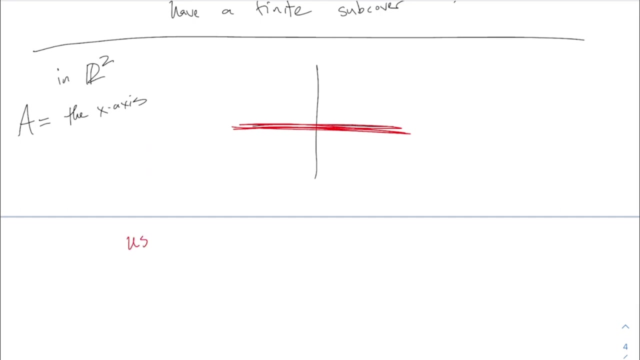 Now, this doesn't even have edges, but that might give you a hint about where you want to put the balls. Any ideas? I have two different natural ideas and both will work. Oops, Oops, Think about overlaying. you know balls on this thing so that it covers every point in a way that you actually need. 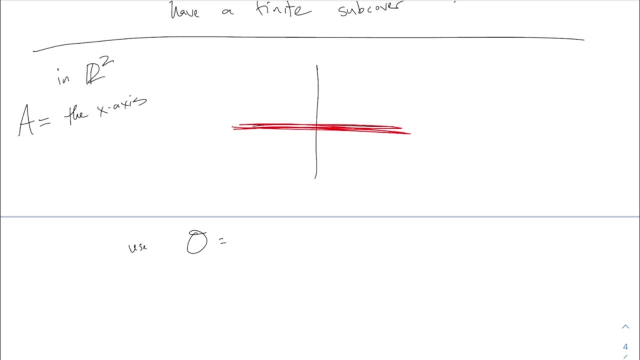 How about infinitely many of them? Yeah, Yeah, I don't know. I was thinking like when it starts long, Start small and get bigger. Start small and get bigger. Yeah, This is one of. I said I had two ideas and both will work. 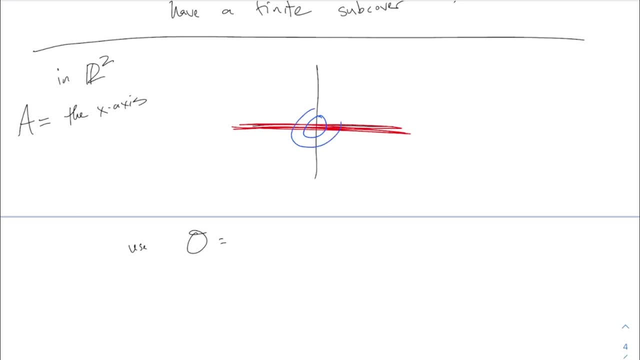 She said: start small and get bigger, like here, here, here here. This, I think, fits very nicely into my general suggestion of making them stretch out to the edges. There's no edges, It just goes out to infinity in this case. 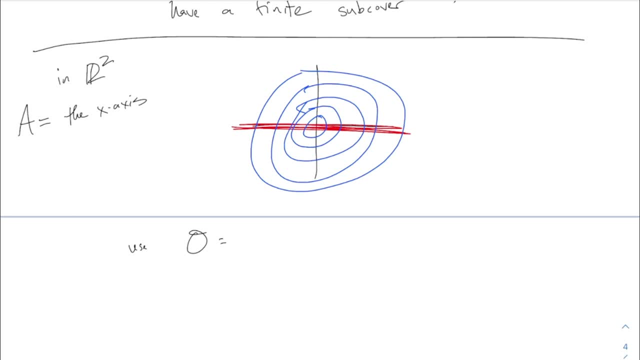 But yeah, if these are your open sets. so the way I would write this is as a set. it's the ball around. zero, Zero, Zero, Zero, Zero of radius n right, That's the notation. This zero is zero. I guess I mean the origin. 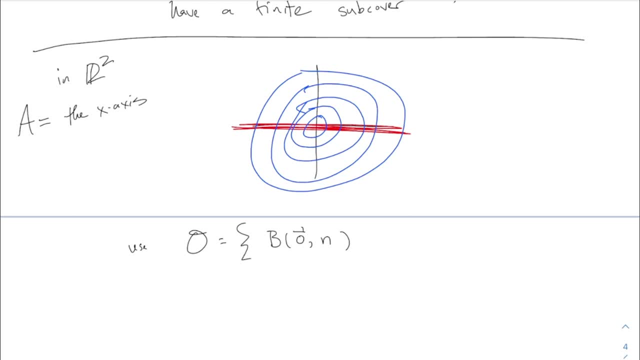 Maybe I'll write it as a zero vector. It's the ball around the origin of radius. You start with the radius one and then radius two, and then radius three, et cetera. These are increasingly large open balls And they do cover the entire x-axis, because any point of the x-axis eventually lies within one. 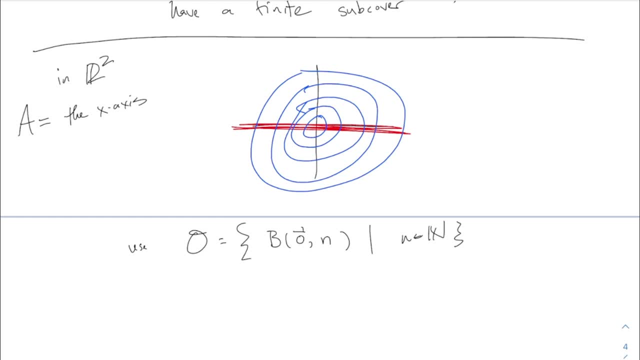 There's infinitely many of them, of course. And then, is there a finite sub cover? The answer is no. If you only take finitely many of these, they're not going to cover the entire x-axis anymore. So this is my open cover. 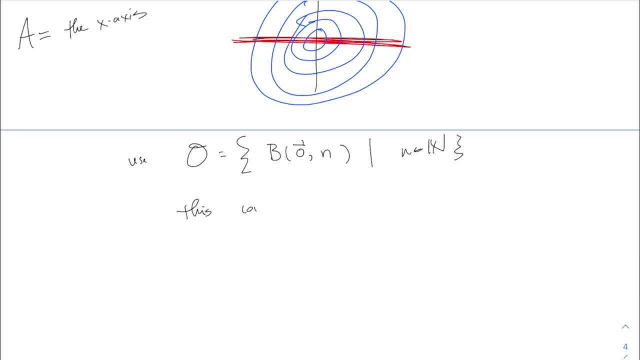 This covers the x-axis, But we need infinitely many to cover it. So there is a finite sub cover. There's infinitely many, But we need infinitely many to cover it. So there is a finite sub cover, But we need infinitely many to cover it. 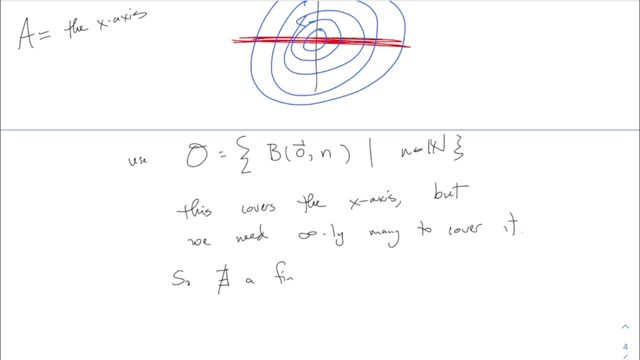 So there is a finite sub cover. There does not exist a finite sub cover. There does not exist a finite sub cover. Great, I said I had two ideas. That was one of my ideas. Anybody have a different idea. You can actually do this using sort of this is using a bunch of balls centered at the origin of increasing radius. 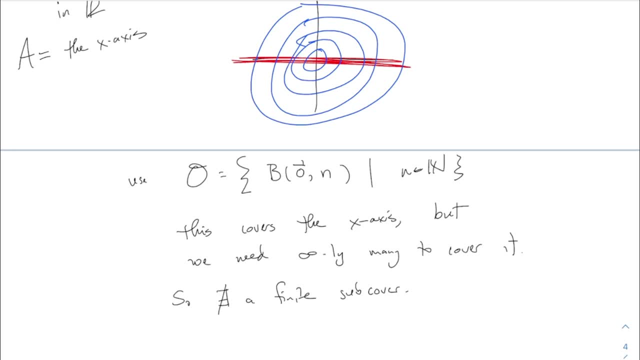 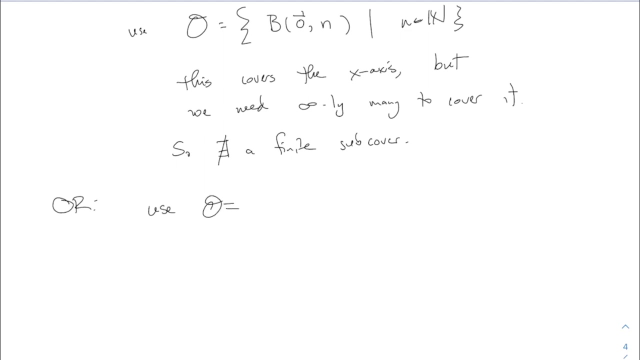 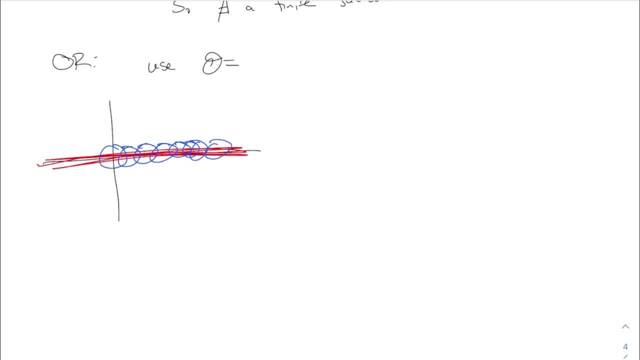 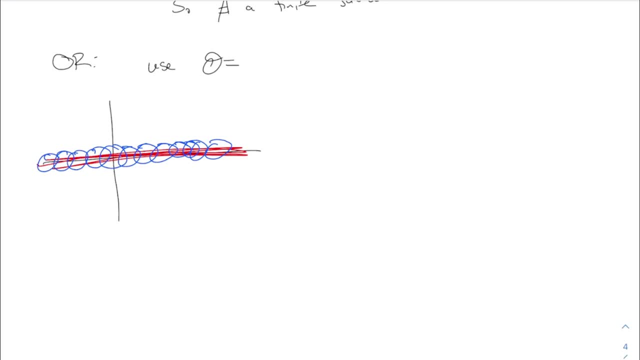 All right, That would also be a covering of the entire real axis: real axis, X axis. In complex analysis, this is the real axis. that's what I meant to say. This will cover all of the X axis And then, it is still true, you need infinitely many of them to cover the whole thing. 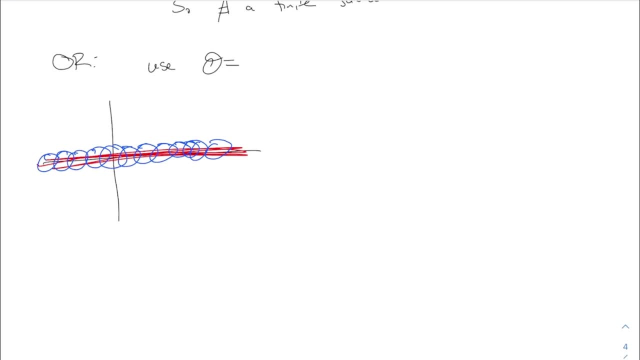 They have some overlap with each other, But you still need one clean sub cover. Okay, So there is infinite sub cover, So there is into them. still need infinitely many of them. so in this case, I would say: the balls that I'm. 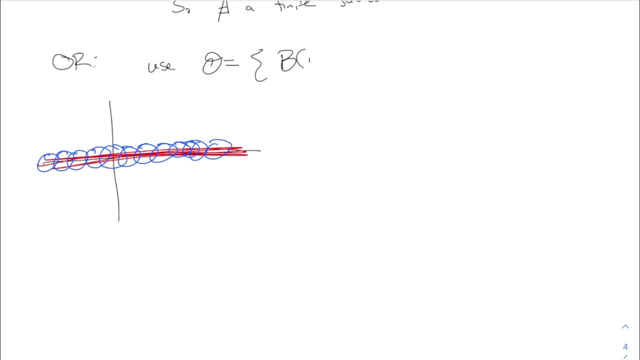 using would be ball around n of radius. I think you have to use two or something like that. that's so that, no, you can use one, you don't need to whatever. I mean, you can use two if you want to. the ball around each number of radius: one. so the 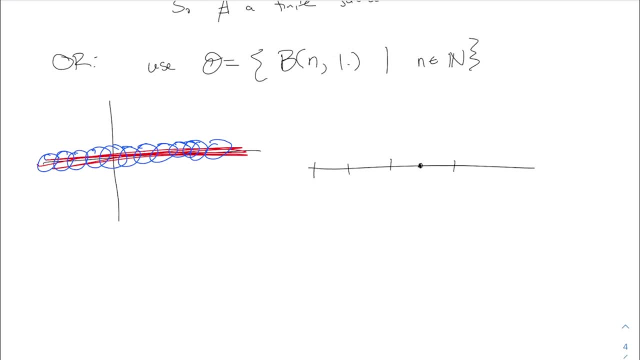 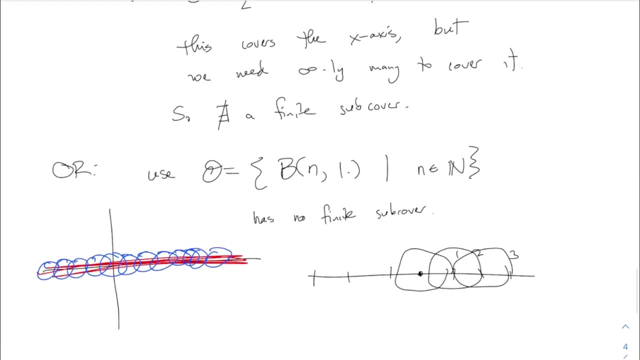 first one, if these are the numbers right- one, two, three- I'm talking about this ball, this ball, this ball and so on. right, that covers the entire x-axis and it has no finite self cover. all right, either way, we'll get the job done. um this, actually, this example here suggests a general fact, and that is, um, I think. 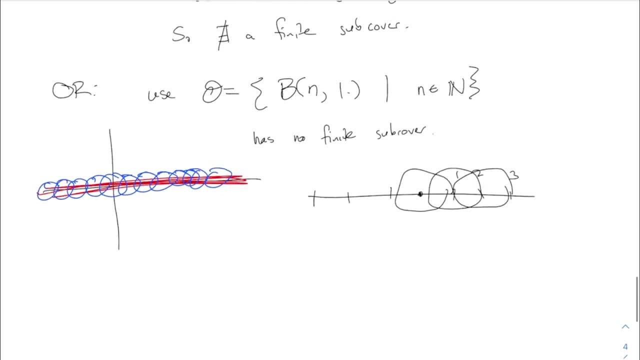 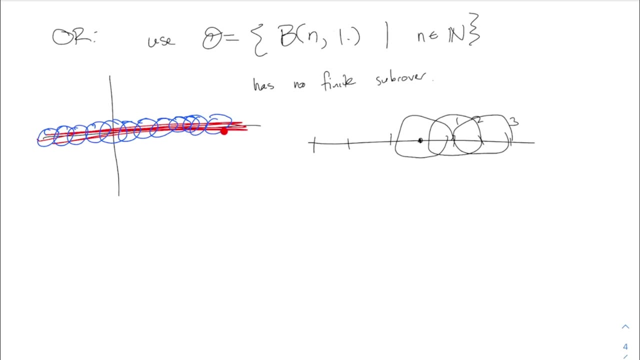 really both, and I'll just- I'll just focus on this picture here. you can do a similar trick on any kind of set that stretches out forever. right, this set if it's, if it goes all the way out, sort of to infinity or something, then you can. 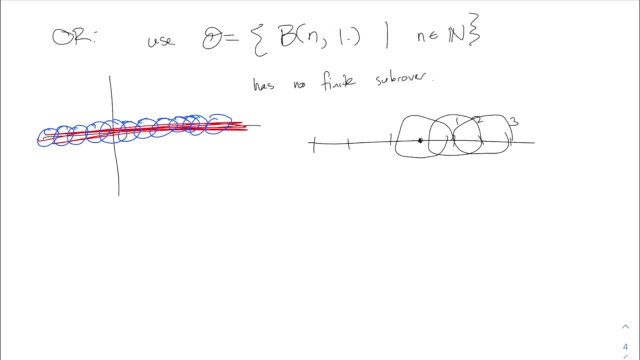 always put these little balls around every point and you're guaranteed that it will stretch out to infinity and that then there cannot be a finite sub cover because you need these little balls to stretch out to infinity. maybe it's actually clearer in this example if the set stretches out. 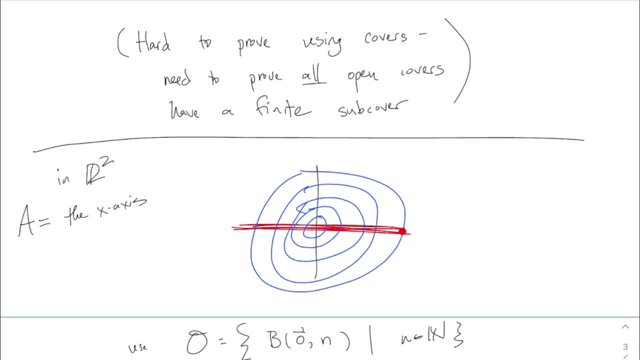 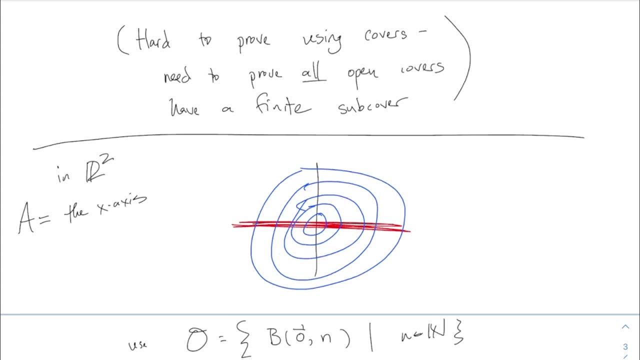 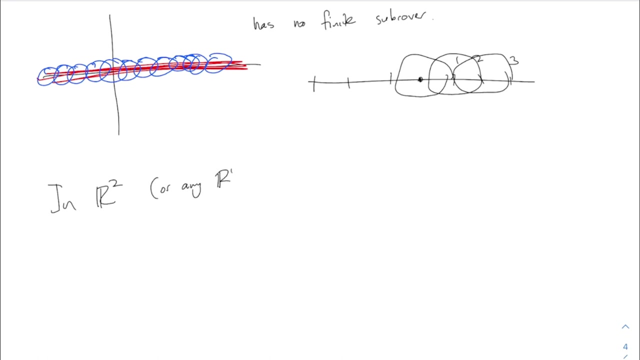 to infinity you can use this covering and you're guaranteed as long as the set stretches out to infinity, you're guaranteed that this does not have a finite sub cover. so I would say in r2, or actually n? e r? n, any set stretching out to infinity. 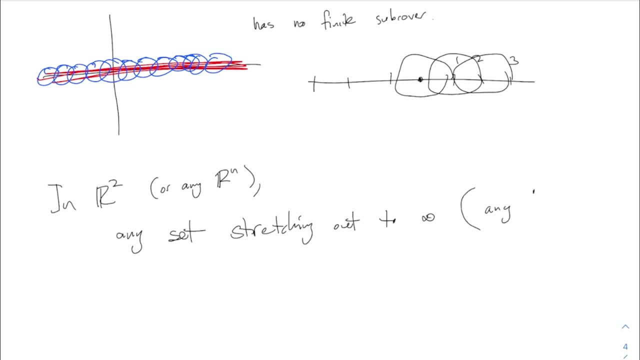 What I mean by that is any. maybe I should have just said it this way in the first place: any unbounded set, Any unbounded set in Rn, you can use that. It can be covered by the first one that Julia said. 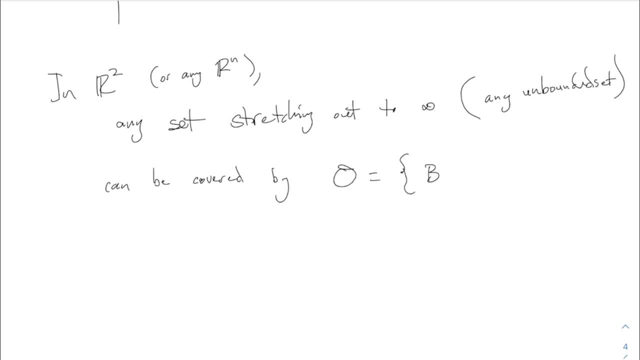 Ball around 0 of radius n. That's this one. No matter what your set is, it will be covered by those circles. Eventually those circles cover- I mean that covers all of R2, so any subset. But if your set actually stretches out to infinity, 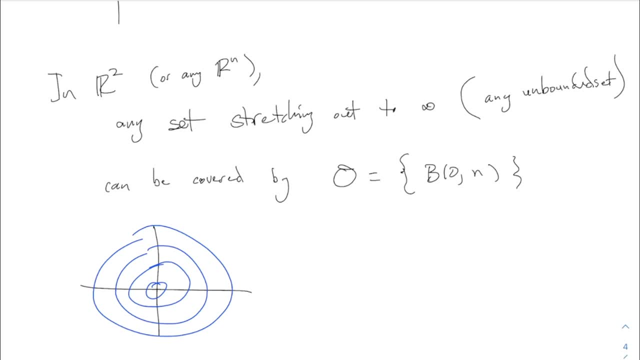 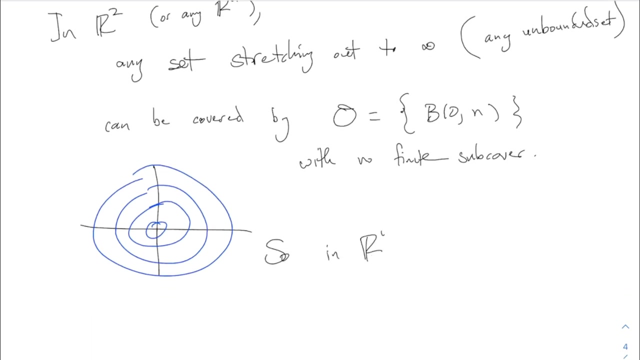 then that means that no finite amount of these can ever cover it. So any set stretching out to infinity can be covered by this with no finite subcover, Alright. so that means in Rn any unbounded set is not compact. 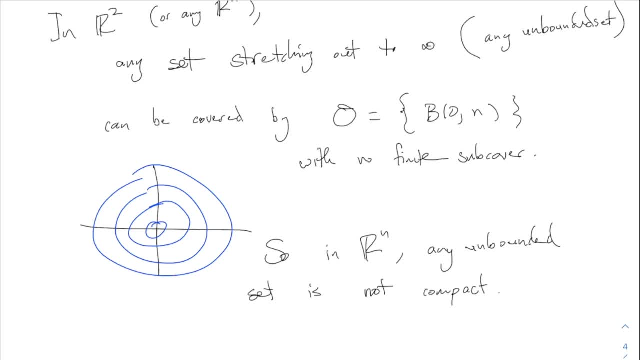 Because an unbounded set you can always use that sort of bullseye type cover And if it's unbounded it means you cannot use only finitely many of those bullseye type sets. So in Rn any unbounded set is not compact. 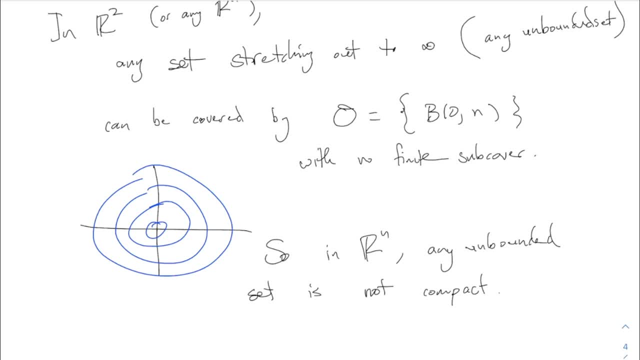 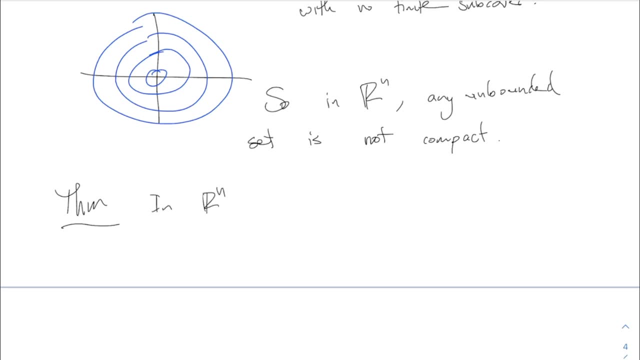 And this actually looks nicer if you write the contrapositive of that. So maybe I'll write that as a theorem In the contrapositive. it says in Rn: compact implies bounded. That's the contrapositive right. 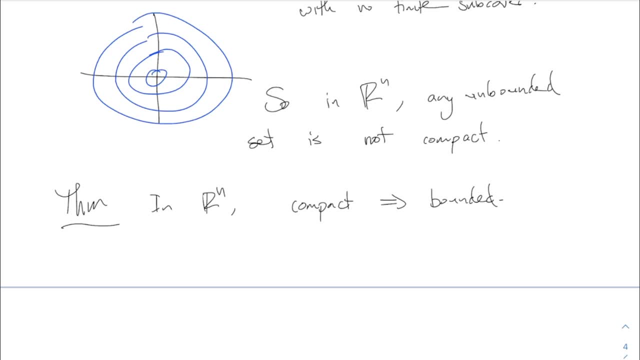 This says unbounded implies not compact. The contrapositive of that is: compact implies bounded. And this is actually sort of half of the Heine-Borel right. The Heine-Borel says compact is the same as closed and bounded. 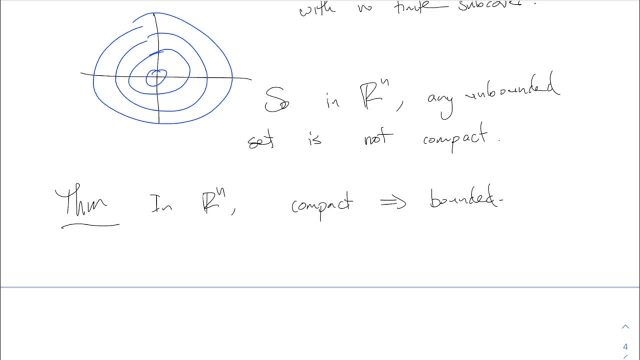 The whole Heine-Borel is a little tricky, but this is part of it at least. Alright, a compact set is automatically bounded In Rn. This only, unfortunately. this boundedness only really makes sense in Rn If you have some other topological space that's not Rn. 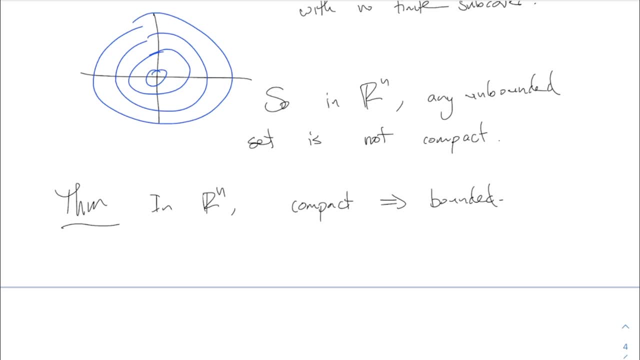 then it may be that you don't even know how to talk about boundedness, because boundedness has to do with distances from the origin and that it's not always possible to discuss in a weird topological space. Alright, I had one more example. 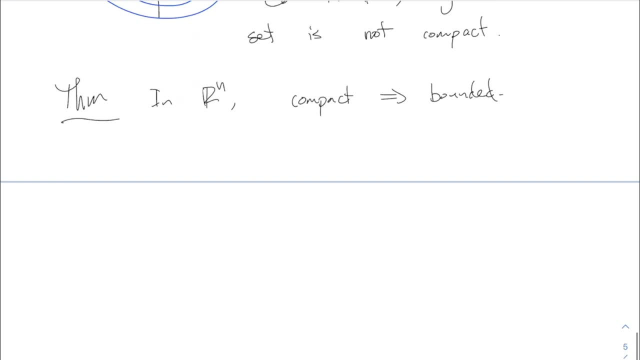 How about another R2 example? And then I have some for you all to try. How about another Another example in R2.. The um, let's try the unit open disk That would be sort of this: set The inside of the circle, not including its boundary. 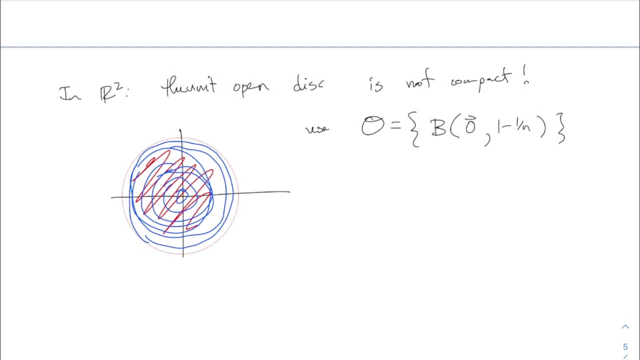 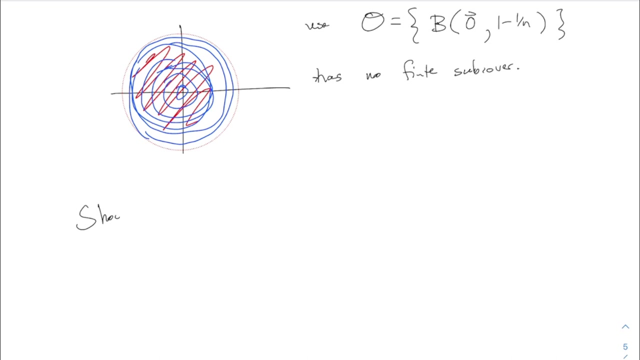 approaching one. yeah, great, this is the unit. open disc is not compact. that is an open cover. and why? this has no finance of cover? great, all right, I got some for you to try. so your job in each case is show it's not compact by you know what. 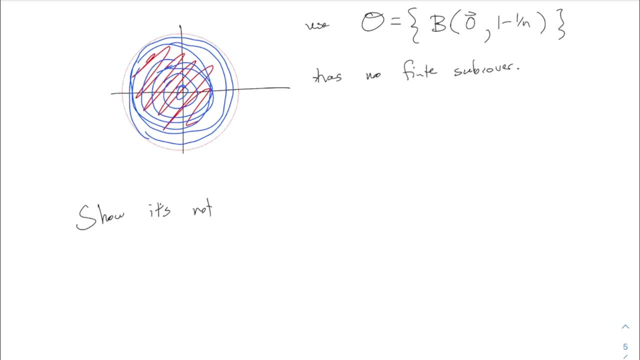 you have to do is you describe an open covering and then say: you know, say that this open cover has no sub cover, so show it's not compact. in each case, as I said before, to show something is compact is quite a bit more complicated and, to be honest, usually 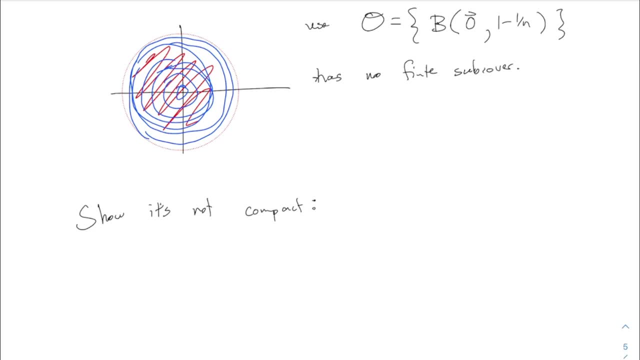 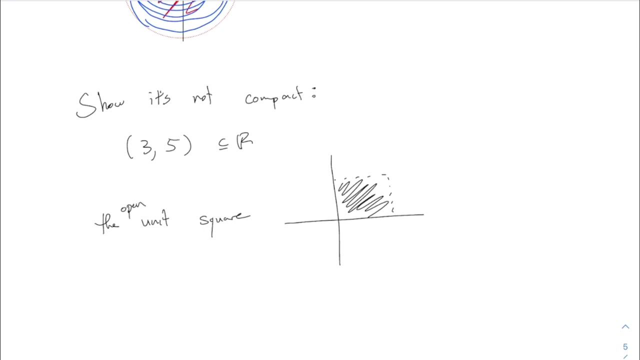 I use the hein hingaburrell's Dim depositing. how about the interval decision from three to five minutes? and how about the interval from two minutes to man's HIM- 것으로 Latinoana and 5 in R? How about the unit square open unit square in R2, like that I mean, for it contains: 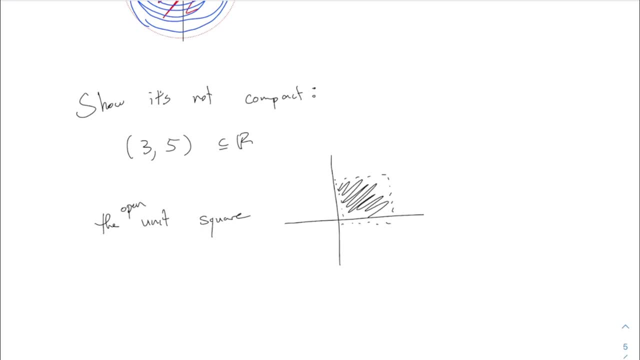 none of its boundary points, but it's just. if you like, this is you could write this as a product: 0, 1 cross 0, 1.. It's a product of two open intervals, The open unit square. 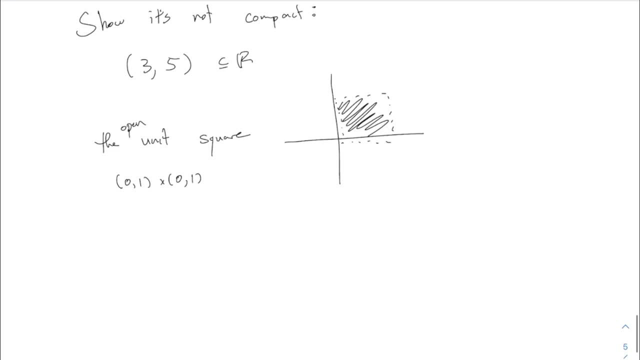 in R2.. And then I got one more, I got two more. I should make them red, since I've been making all my other sets red. This is in R2, sort of a cross, a horizontal interval and a vertical interval, just kind of the union of. 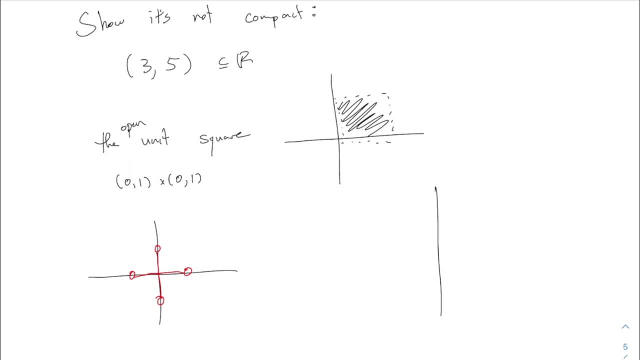 A horizontal interval and a vertical interval, And then the last one. This last one is what they call a punctured disk. It's a closed disk, so it has its boundary, although that's not really important. What's important about it is the puncture that is. 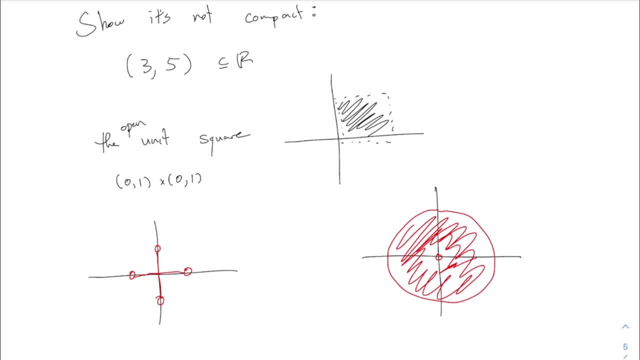 this does not include the origin. It includes all the whole disk, but it's missing that one point in the middle. That also is not compact. All right, see what you think. I'll give you a few moments. We got about 13 minutes remaining. 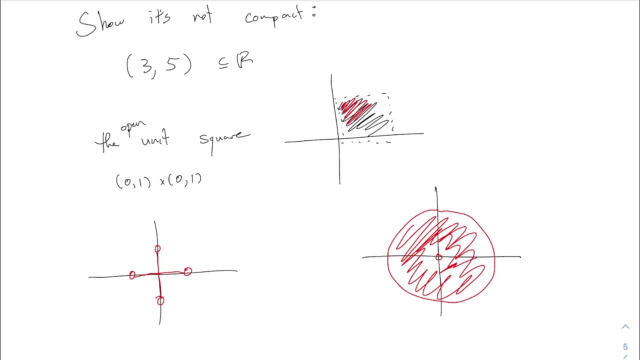 so maybe we can work on these for a few and then we'll talk about them. I think that last one is a little tricky. The other ones well, they're all a little tricky until you get used to it. Okay, so we're going to go ahead and get started. 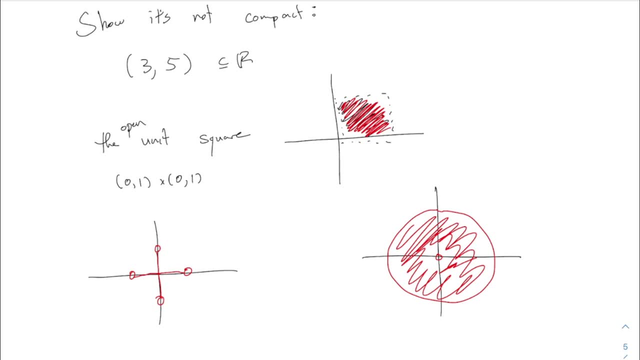 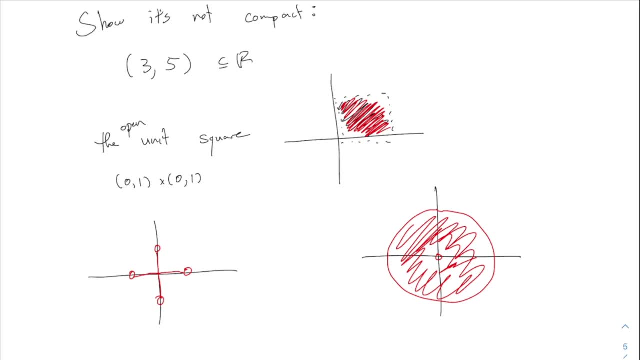 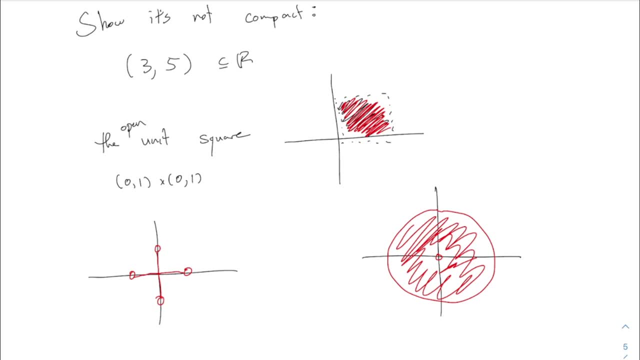 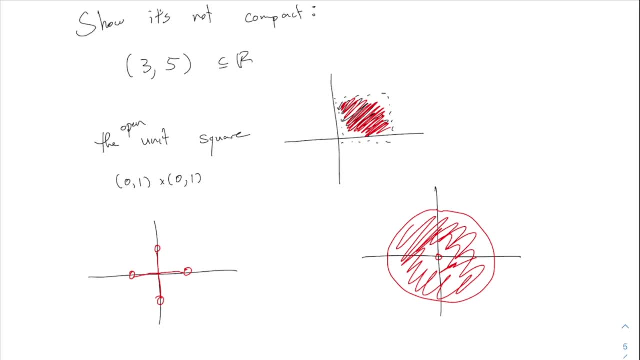 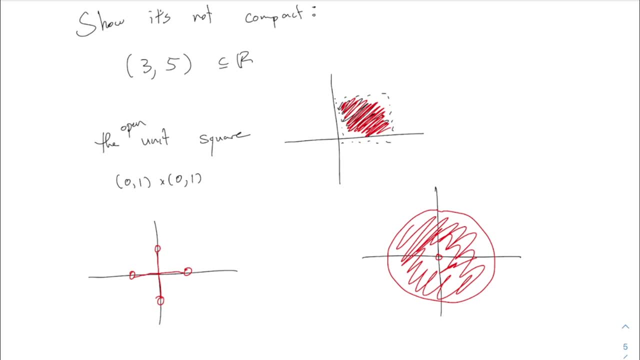 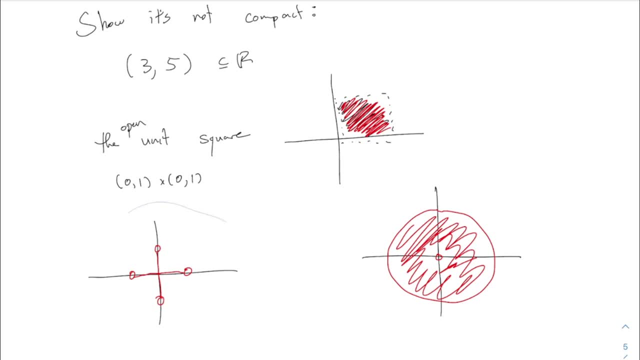 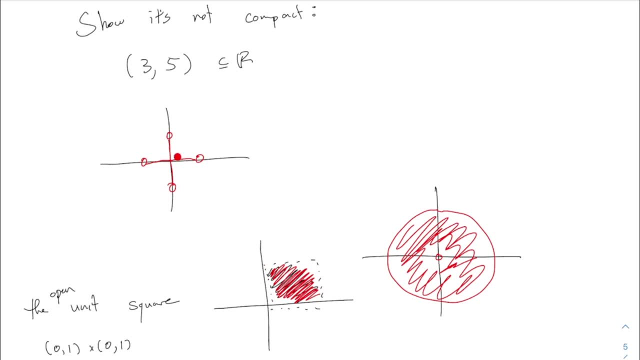 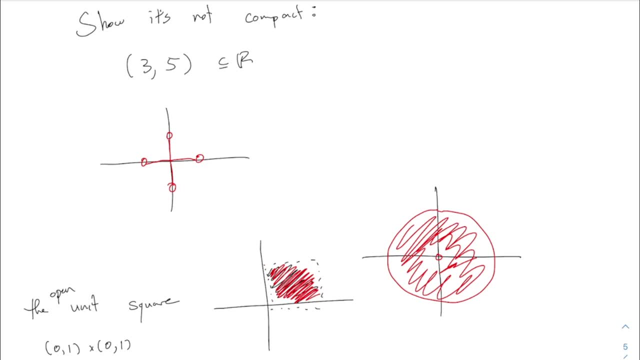 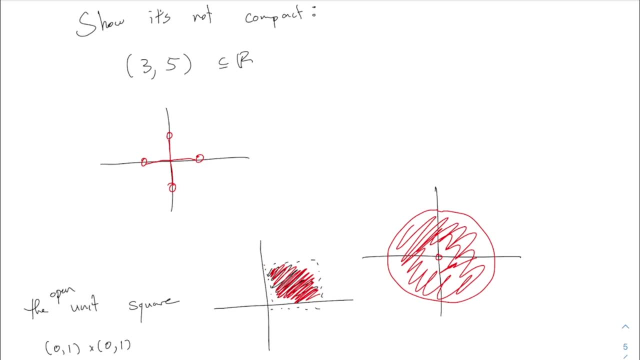 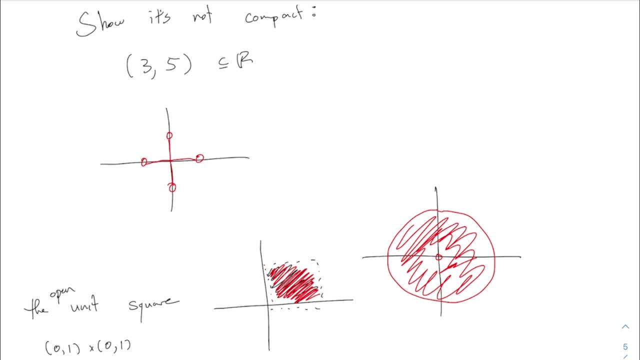 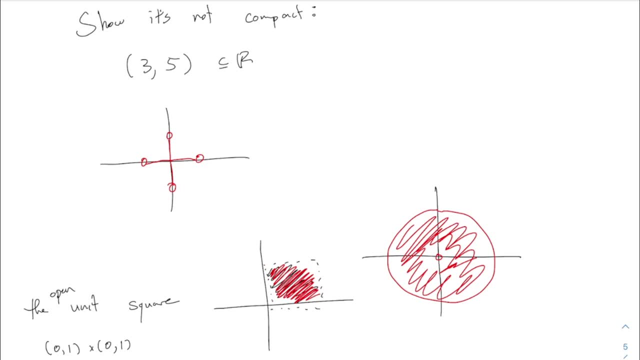 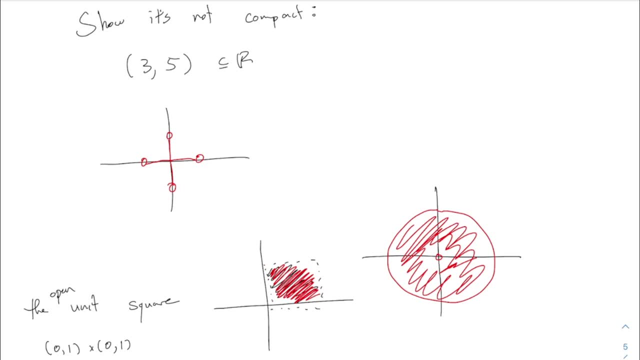 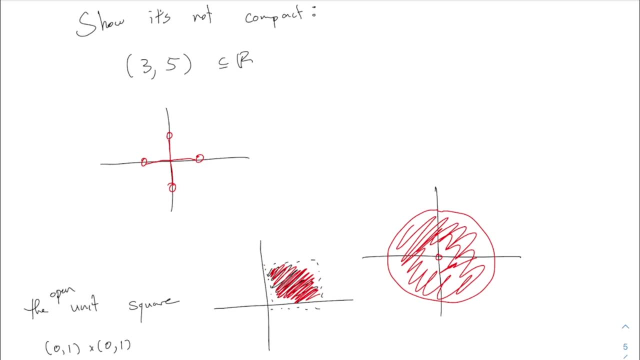 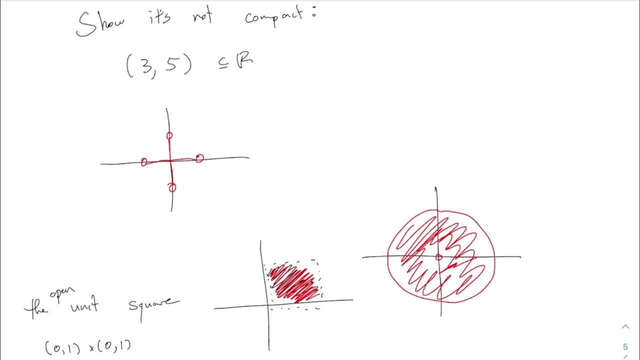 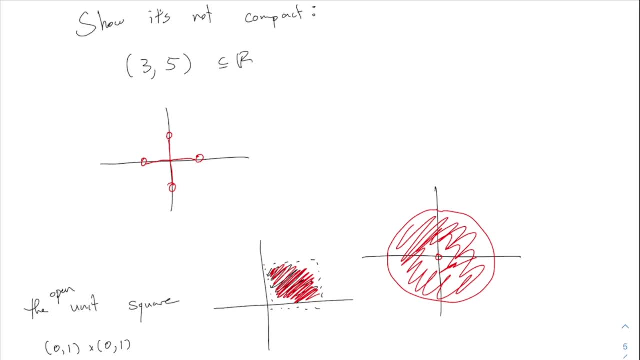 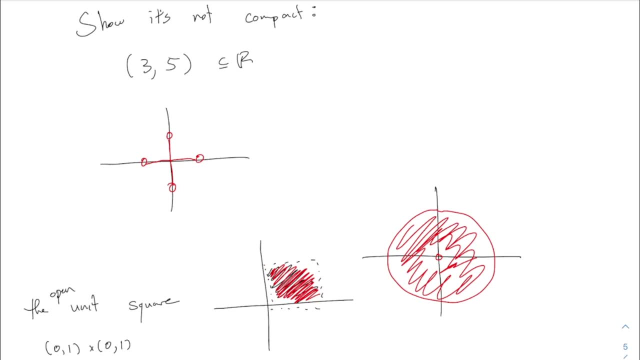 All right, so we're going to go ahead and get started. All right, so we're going to go ahead and get started. It looks like everybody thinks the square is easier than the other one, so that's fine. This happens especially the first time I teach a class, which is the first time I've taught. 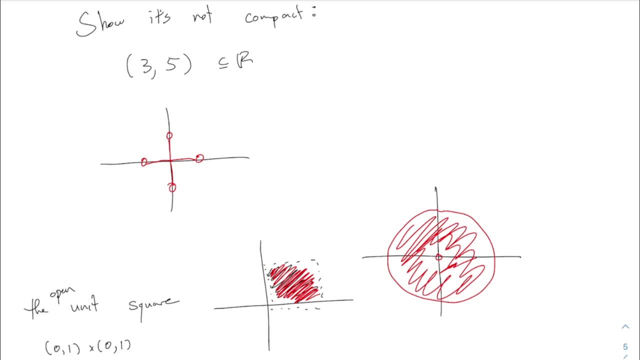 this class. A lot of things that seem obvious to me aren't that, and things that seem obvious to you are not obvious to me, and the other way around. We're all God's children just trying to get by. Yeah, let's say it goes up to one each time. 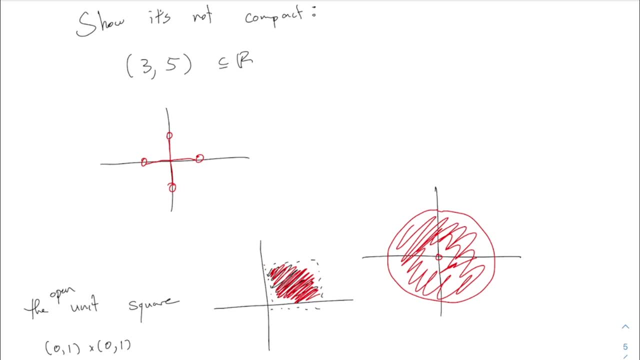 Yeah, Okay, Thank you, Thank you, Thank you. Well, this one is just one of these, right? Yes, Yeah, But then this one, Yeah, This one, But this one is not including zero. Yeah, So for that one I would say it's best, it's easiest to use sets of John Ott balls. 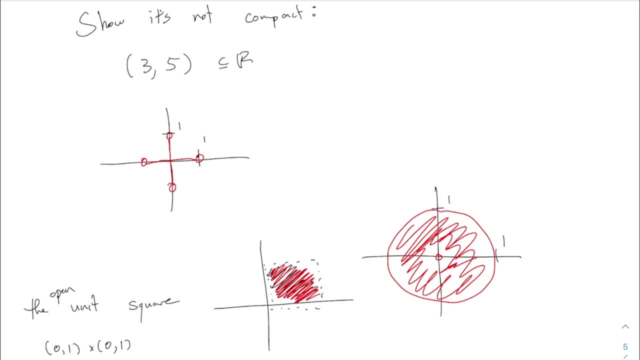 Some other kind of insect. You know another shape: Round, Don't use square, but not a ball. No, there's a square, Okay, So for that one, it's not including zero, Okay. Then we have a set of these others. 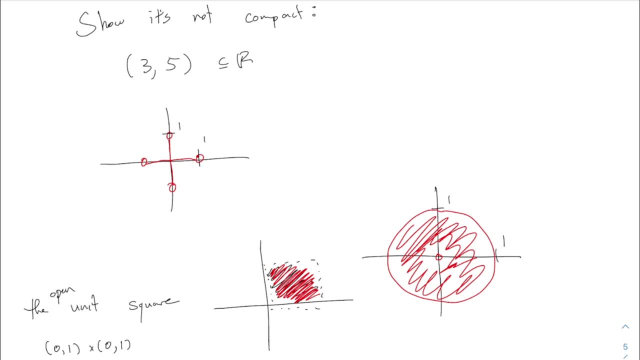 So we just have to make sure that they're not including zero. Also for this one, like I mean, the two myself are not required, but they're also not on the same set. Like the two sets are actually use, They come in different sizes. 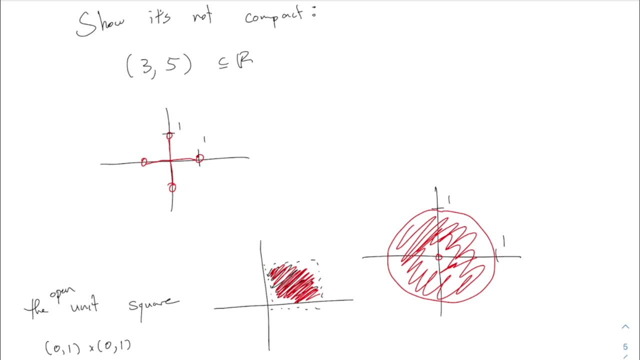 Right, I see. yeah, They're neither the fourth or sixth or the ninth or the fifth. The sixth, The second, I mean they're not included. Oh okay, And so this one is an ink, Oh okay. 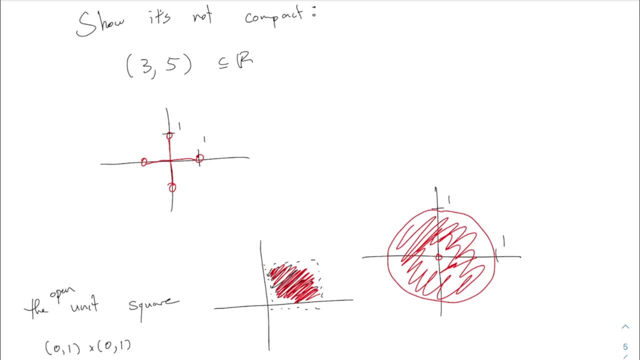 So for that one I would say: it's good, Not a, not a ball. A ball can set anything, basically any kind of shape, without, without its boundaries, That's. that will make anything set, obviously, Um, like saddles. 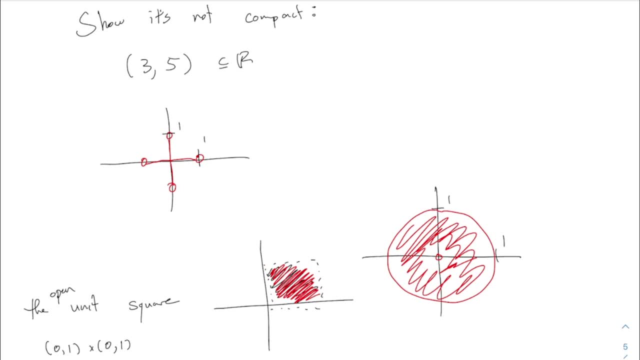 Um, so, such as you're asking, like how they raise, I mean the radius- You could you could say that the radius is usually how they raise the ball, And then you could say: it has the ball raised, which means the ball raised. 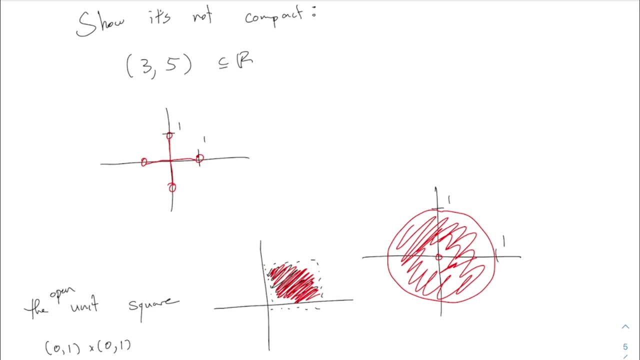 Yeah, And then you can just draw it out so that they're the same size. It's just not the same. That's interesting. What are you supposed to say? It's just that they're not the same, right? Right? Oh, it's not the same. 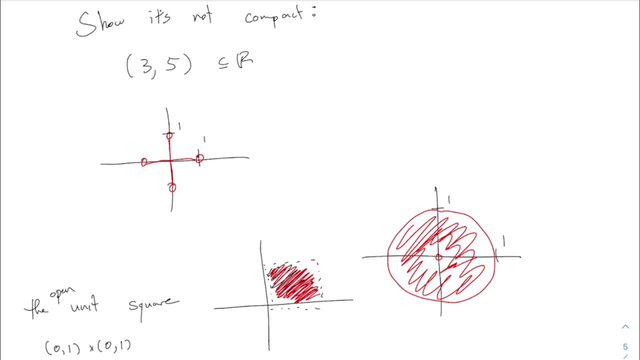 No, No, No, It's just not the same. No, it is. It's really not the same. No, it's not the same. It's too long, so it's not the same. And then it's just not the same. 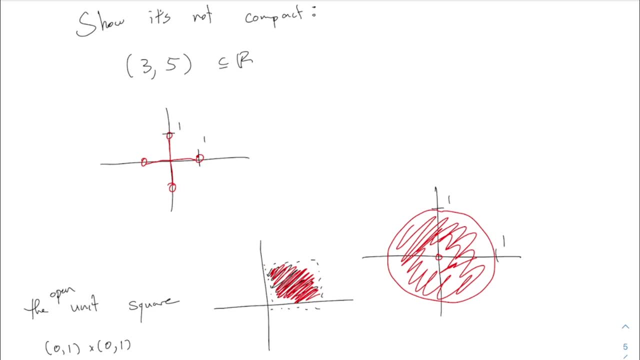 Mm-hmm, I like that. Yeah, Thank you everyone. Okay, And I'm going to set this back right. Is the boundary? Yeah, Outer boundary is I can't remember, but what's that called Yeah. 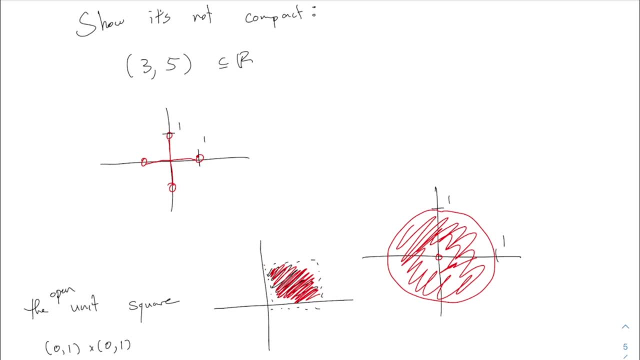 Outer boundary is What's that called? The? Oh, the center, Yeah Yeah, The outerm, The, And you If the, if the, OK, So then there's the. Then it goes this way: 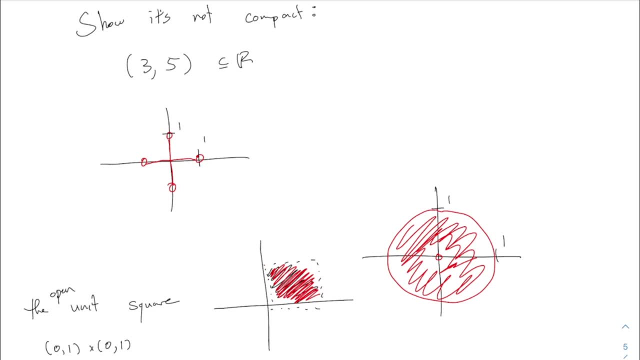 Girls gonna stand right, Right, right. So you'll write hope right here, At the right, right here. Now you wrote That's a little bit specific. I'll give you one more minute and then we'll talk about it. 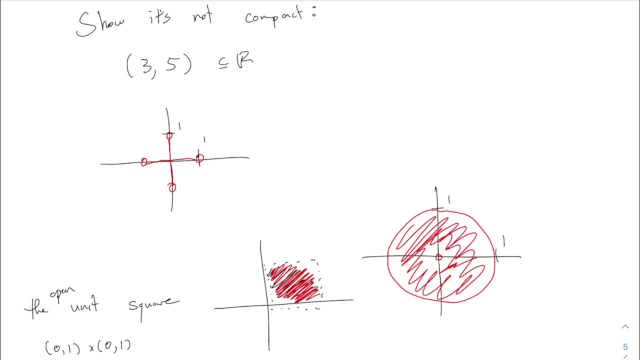 Generally you make shifts, which sort of stretch out tilt, so then you do this one. Oh right, it's not one of those. Oh, you go across this. okay, That's fine. That's actually not this, it's this cross. 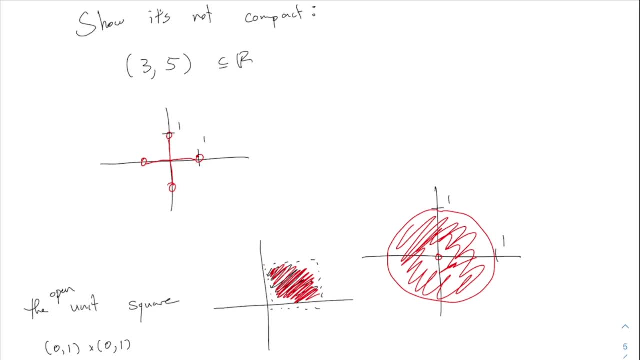 That cross. it's something like a box. Actually, that's the worst. So you know, this box is, which is still fine, and it's the worst. So I would say here, you know what? it's a little bit of a jump, but in this it's. 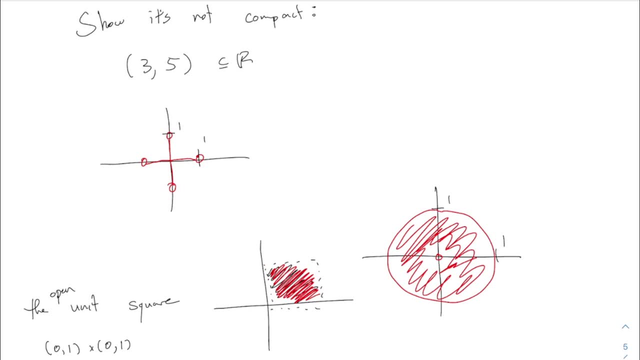 a little bit of a twist in there, right, Right, Because if you wanted to approach it that way, it's a little bit of a jump. All right, I think we've got to talk about these. So people did great on the first one. three, the interval: three to five. 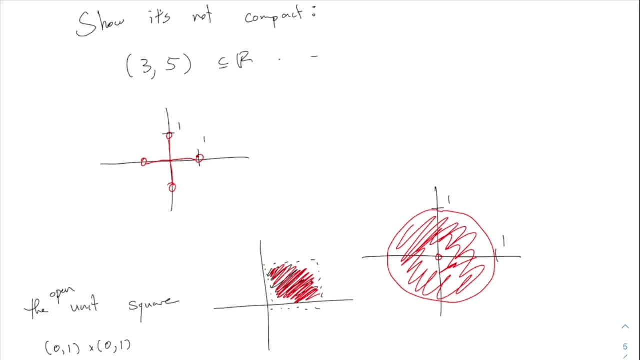 Here I would use the open cover, something like: oops interval three to five minus one over n. This makes it so that The right end point of these intervals approaches five. So I saw some slight variations on that. You could do three plus one over n to five. 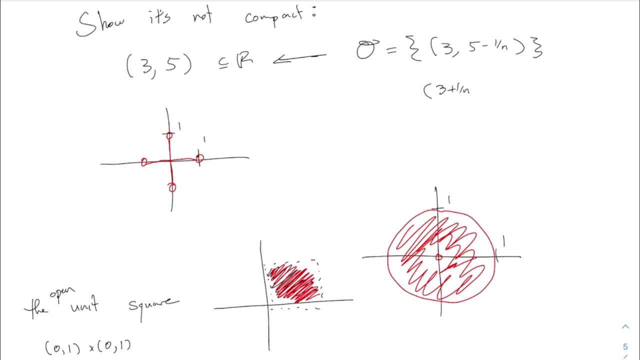 I don't think anybody did that, but that would also work, right? This one would: everything goes all the way to five, but then the left side approaches three, Or you could even if you want to be super fancy about it: three plus one over n five. 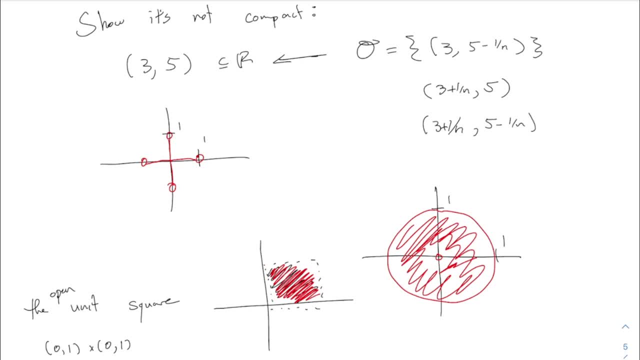 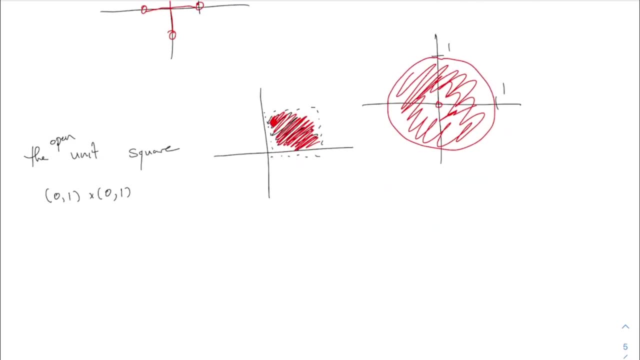 minus one over n. This makes them grow, doesn't matter. both ways, whatever, I would say the first is the most important, Okay, and then the square. All right, people said: this is a great idea that everybody had that. somehow I didn't have. 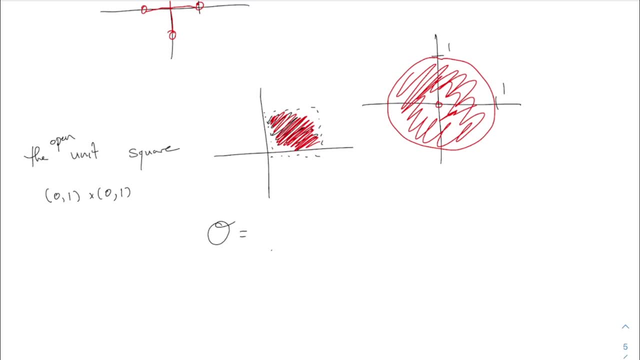 They use. the open cover was a product zero to one minus one over n cross. zero to one minus one over n. This is great. That is this would look like on the picture. it would look like open boxes, Open boxes. 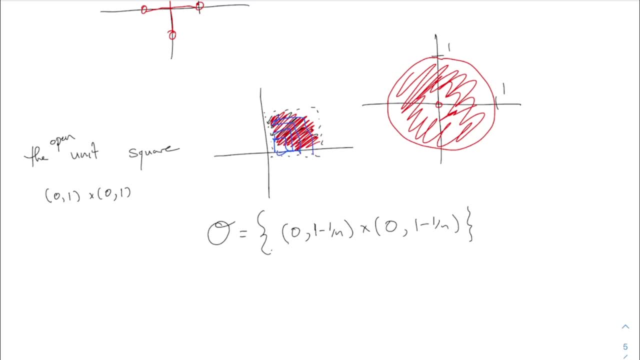 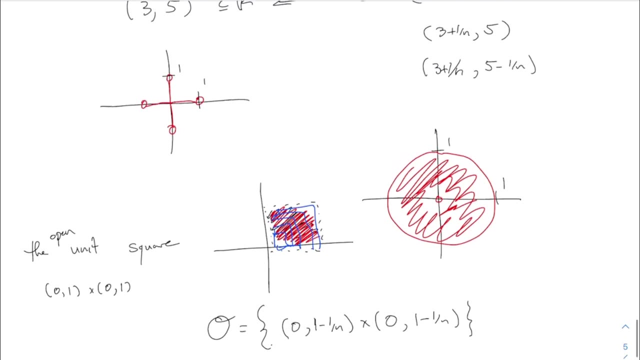 Open boxes that are getting bigger and bigger, approaching out to the edge right. Excellent, The cross up there. there were a few answers that I saw, but I think most people ended up just using the ball of radius centered at the origin of radius one minus one over. 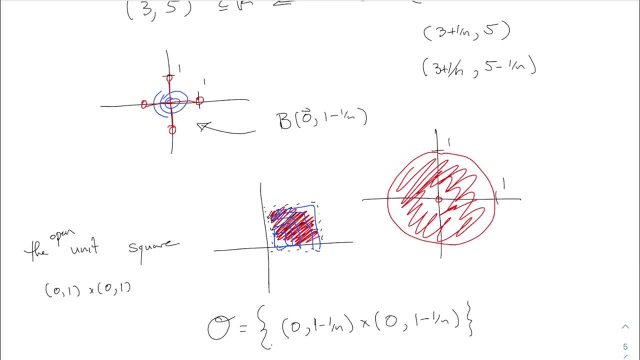 n. This makes this kind of bullseye style balls which are approaching those four points, And that's all you need. You could also use. I saw some people used boxes like rectangular boxes. That would be the interval minus one, minus one over plus one over n to am I doing that? 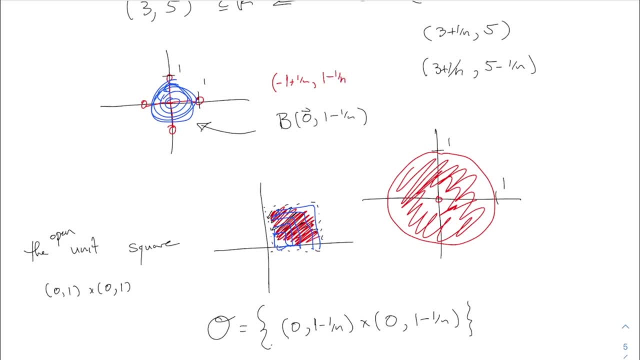 right, Yeah, One minus one over n, something like this. And then the same thing again. This will make squares That go like this Eventually approaching. you know this set that you're looking at. right, Same idea, using boxes instead of circles. 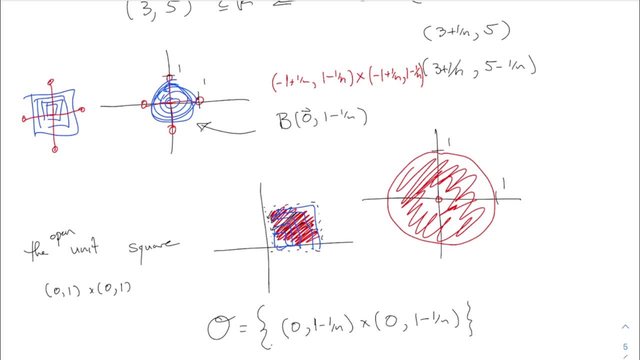 That would work. also, My idea for this one. actually, I thought this was, this was going to be like a tricky, a tricky, tricky, cute example, And everybody came up with a, with a much simpler solution than I had in mind. 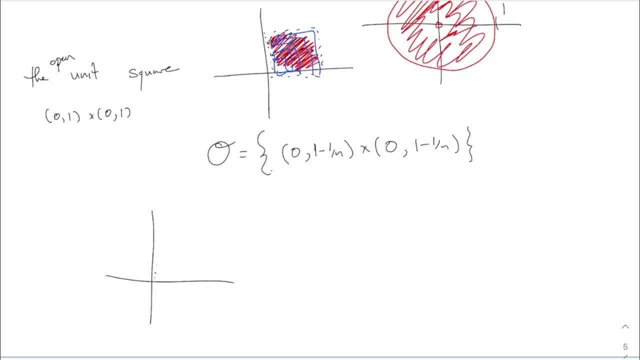 The. what I had in mind was- Let's see if you think this is cute or stupid. This is my original set. I used the same bullseye thing with radius approaching root 2. And this covers the whole square, but approaching that corner point. 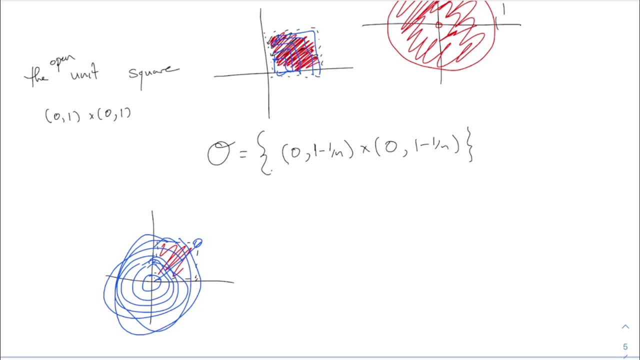 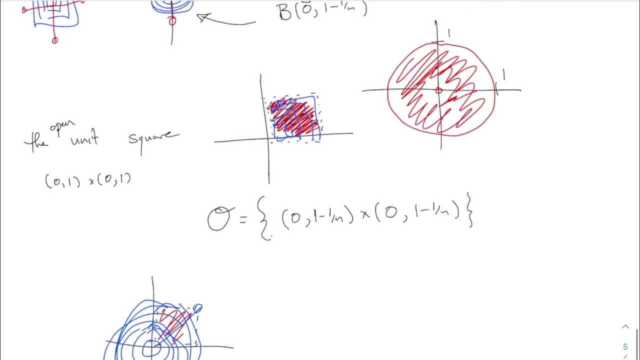 And so you need infinitely many of those sets. Are you impressed, or do you think that I'm being needlessly complicated? This seemed obvious to me because I had just done this one and I realized: oh, I can just do the same thing again, and it will still work. 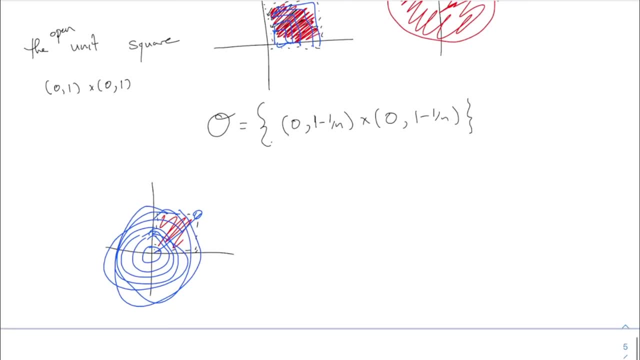 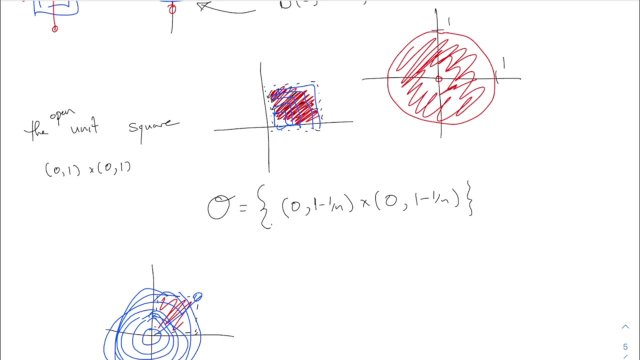 And it's true. You can just do the same thing again and it will still work. You have to stretch the radius a little bit, All right? What about this one? This one is more interesting, maybe because my hint that I gave to everybody is: you can't really use ordinary balls as the whole set. 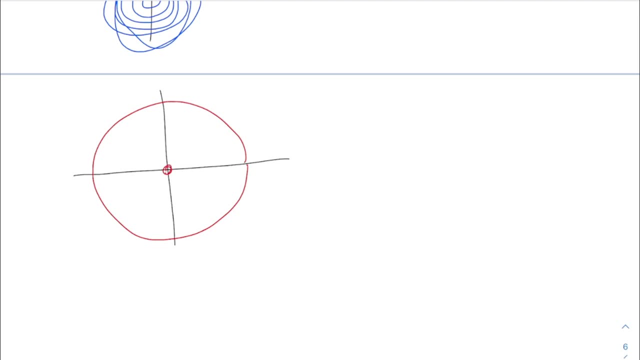 because an ordinary ball will have the same center point in there, certainly if you take a ball centered at the origin. Oh sorry, It's time to go. What some folks came up with was sets that look like sort of a donut-type shape. 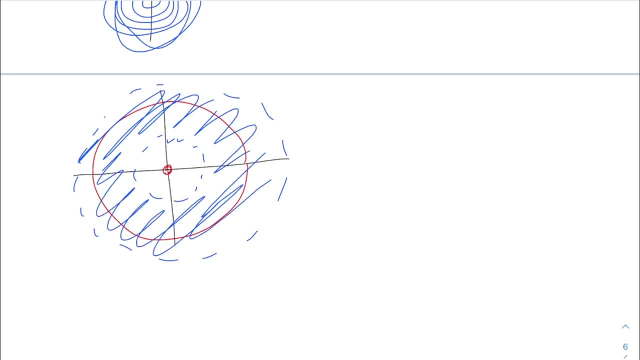 This is called an annulus. All right, That is like that. and then you make it so that this outside radius stays like it is every time, but the inner radius You go down the sequence of sets approaches the origin, And the cutest way to write this would be: what I have written here is something like the ball.